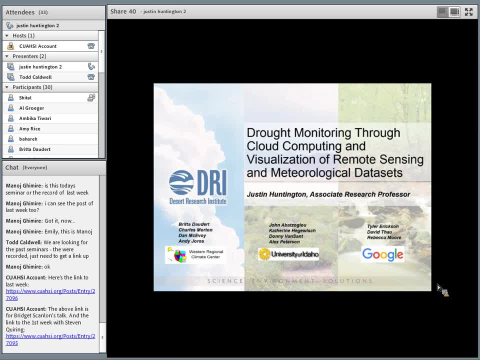 thank my collaborators on this project, a host of folks from DRI and the Western Regional Climate Center and John Abatzoglou's lab at Universe, Idaho. They've been really instrumental in everything I'll be talking about, And then, finally, our collaborators at Google, who 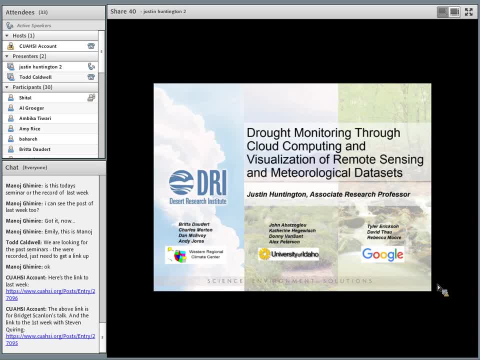 really helped us get this cloud computing project going. Thank you, Thank you all, Thank you everyone, Thank you, Thank you everyone for joining us, And I'd like to thank our panelists, the team at DRI, for their work off the ground that. 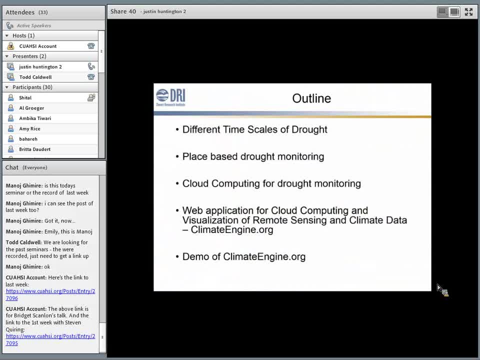 I'll be talking about. So, just for an outline, I'm going to be talking about different timescales of drought and then place-based drought monitoring, and then how we've gone with cloud computing for this place-based drought monitoring as well as regional drought monitoring, and then talk 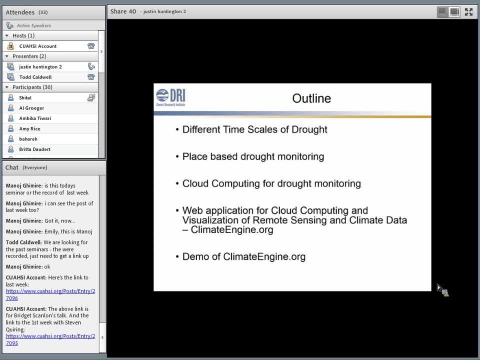 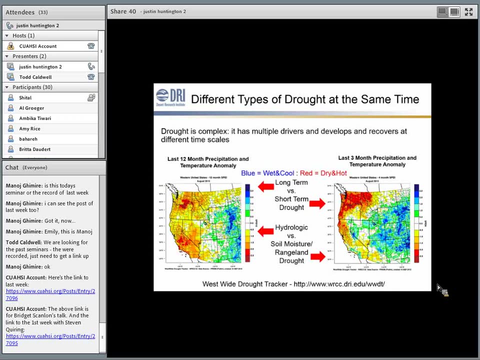 about the location that our groups at Universe, Idaho, and here at DRI have developed called ClimateEngineorg. And then, finally, I'll do a couple demos of ClimateEngine. So, first off, drought is pretty complex in that it has multiple drivers and develops. 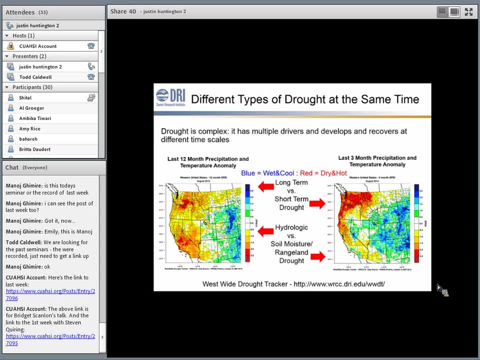 and recovers at different timescales, And so you can have different types of drought happening at the same time, And so on the left. here is basically the last 12 months of precipitation and temperature. It's this combined index called the Standard of Precipitation Evapotranspiration Index. 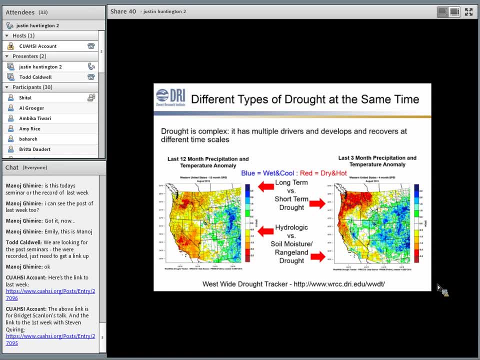 So it combines both temperature and precipitation characteristics And so you can see, over the last 12 months, all the red areas showing the current western drought, which is more of a long-term or what we would call perhaps a hydrologic drought. And on the right here are the last three months. 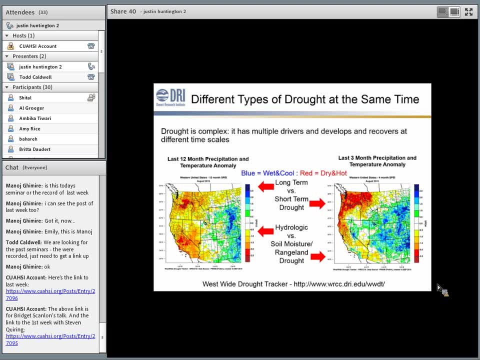 And then on the right, here are the last three months, And then on the right, here are the last three months: Precipitation temperature or SPEI anomaly for August. three months leading up to August And you can see that Nevada, Utah, a lot of the central western states have been exceptionally. 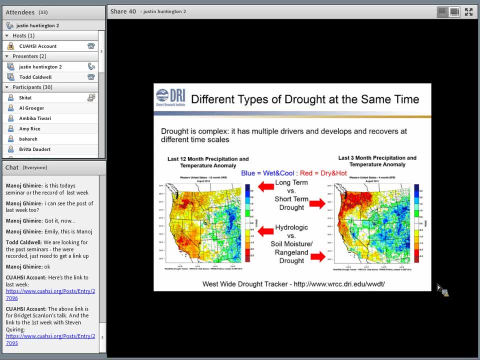 wet, And then we have the Pacific Northwest, which has been exceptionally dry, And so this shorter-term drought or soil moisture-type rain. we're seeing a lot of precipitation and temperature-type rangeland drought is happening at the same time, where we have 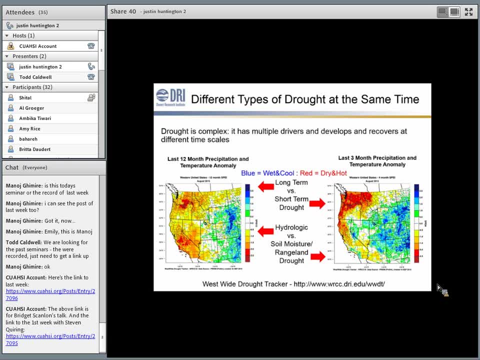 the hydrologic drought, So we can have wet rangeland conditions on top of very dire hydrologic conditions, which is basically what we have now. And these maps were with the Westwide Drought Tracker, which is hosted here at the Western Regional Climate Center and put together mostly by John Abatzoglou and others here at DRI. 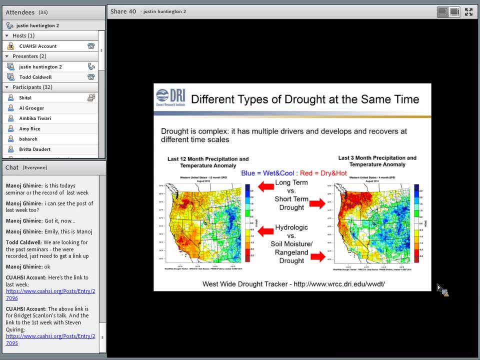 And what we wanted to do was kind of make this process more dynamic and more live, more real-time. These get updated about once a month And we really wanted to be able to zoom in and really focus on, say, particular mountain ranges, particular farm areas, and pull out time series and have it be more up-to-date. 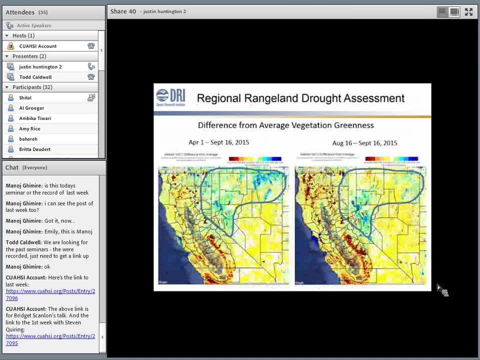 So I'll talk about that here And just a little bit So. for regional rangeland drought assessments, this has been a really big deal this last summer. Here is a difference from average vegetation greenness derived from MODIS NDVI, the Normalized 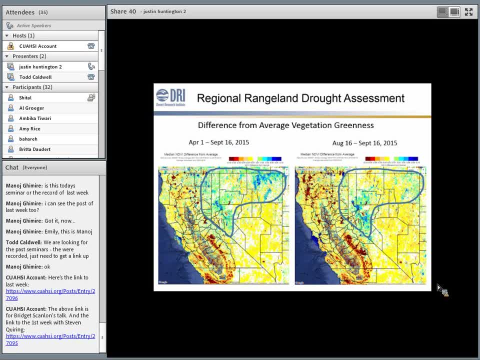 Difference, Vegetation Index And so on the left you can see April 1 through September 16 median NDVI difference from the average, where the climatology is the following: This is the être faible of the 2015 April 1 through September 16th climatology. 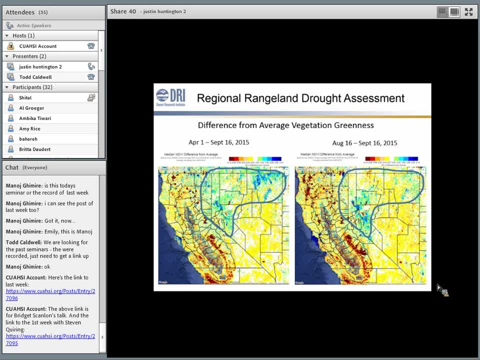 And you can see that in Western and Northeastern Nevada we have abnormally green conditions where vegetation vigor has been anomalously high due to the pretty and summer that we've had. And on the left here, Male Speaker 1, is August 16th through September 16th. so basically what I want to point out is: 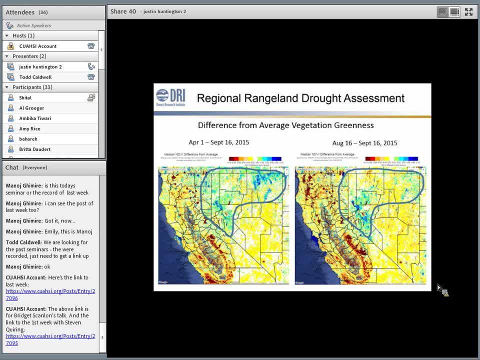 that you can go from being abnormally green to abnormally dry very fast. so basically, the vegetation dried out very fast and some folks might. it's a flash drought. but in in the desert, you know, the flash droughts are real common. this is a real common thing. that can occur if you have a wet spring and then it goes. 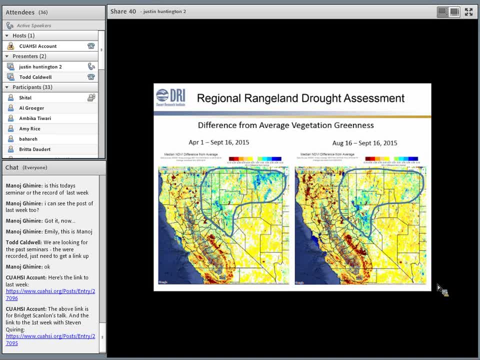 back to normal conditions in the summer, which means that we don't have any rain and and so if we have a wet spring and early summer, like we've had, you can have exceptionally good forage on the range the. the ranchers want to get out there. 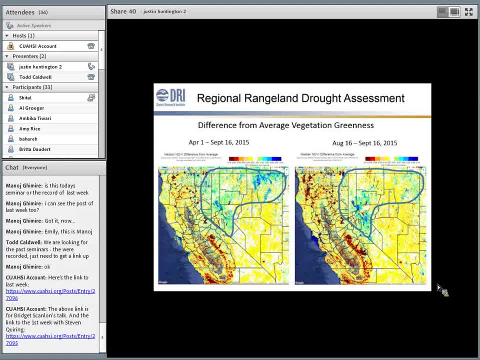 and put their cows out because the feed is great, but yet the UN. so the cattle have not been allowed on the range, even though the forage has been really good. however, that said, the forage dried out exceptionally fast and over the last 60 days. so just something to consider. With these NDVI anomalies, you can 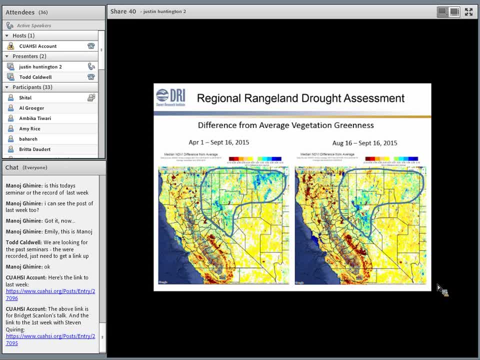 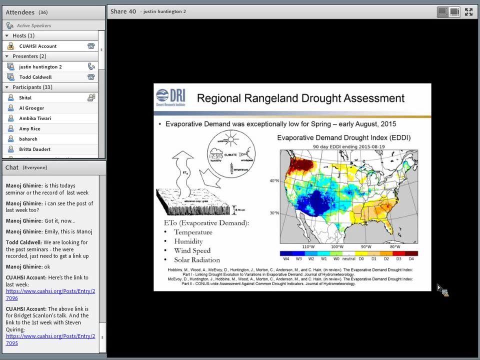 see clearly in California the impact of the drought, all these big red blobs or fire scars, and so that's pretty neat that these all pop out. So, as I was suggesting, we've been really wet this last spring and summer in the Southwest. 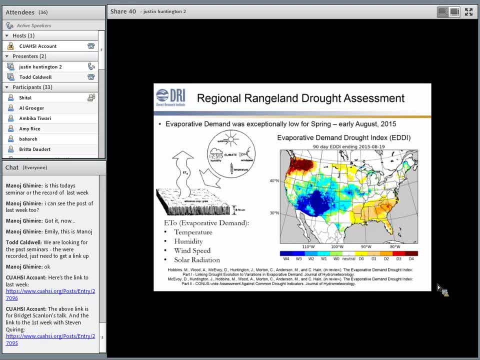 and this is a new index that our group created called the Demand Drought Index. It's basically anomalies in reference ET, physically-based reference ET, based on the Pimmel-Montith equation, and so this is the 90-day Pimmel-Montith equation and this is the 90-day Pimmel-Montith equation. 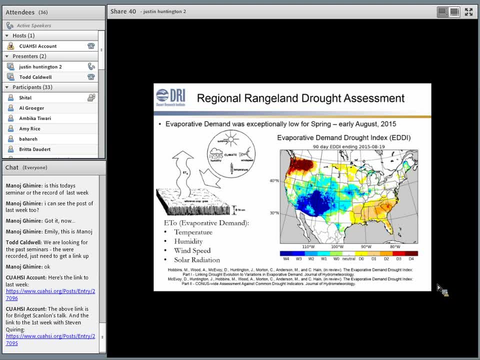 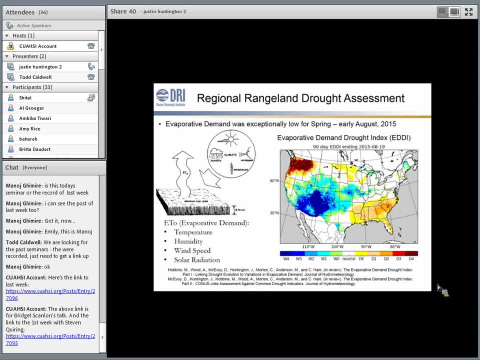 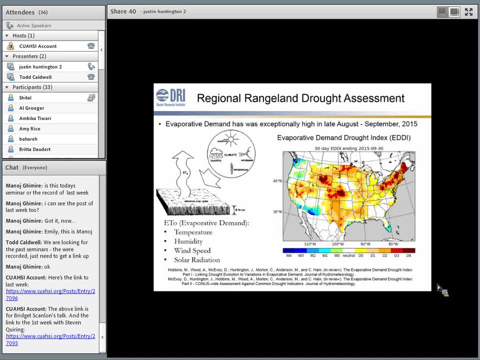 so clearly showing those wet conditions that I was alluding to earlier. And then here's basically a 30-day ET ending in September 30, and so you can see how the mid-summer period has been quite warm and that anomalously high evaporative temperature. 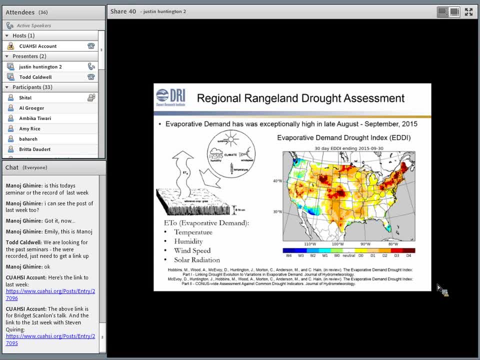 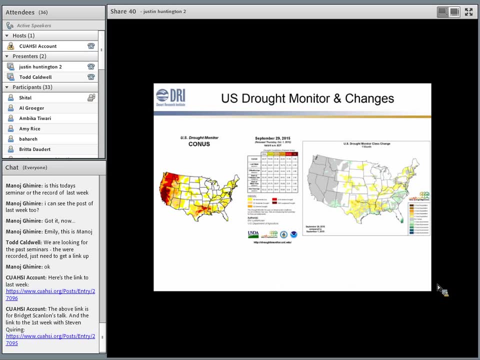 and evaporative demand basically caused all that vegetation that I showed earlier to dry out exceptionally fast. So a lot of this is tied to evaporative demand in terms of how things change rapidly. So I just wanted to talk about that a little bit more. how we can use these multi-scalar. 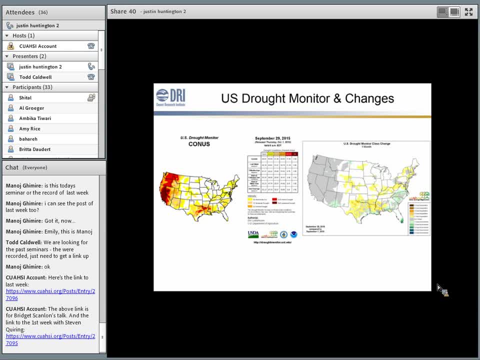 drought indices to dig in and look at changes and how multi-D in terms of changes can show something change using remote sensing, whereas the US Drought Monitor map is generally more of a hydrologic type driven drought indicator. And so here's the map released on September 29 showing, of course, drought conditions. 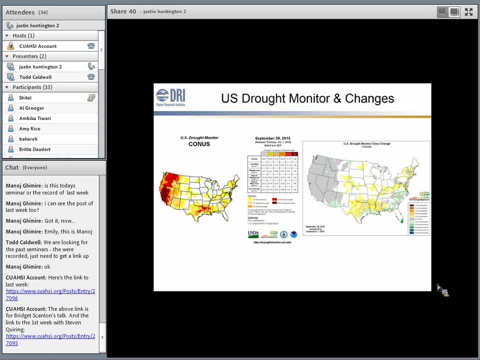 over much of Nevada and, of course, California. And on the right here is the change for the last month, well, ending at the end of September. So it's a one-month change map ending in September, end of September, And you can see that the map hasn't changed. 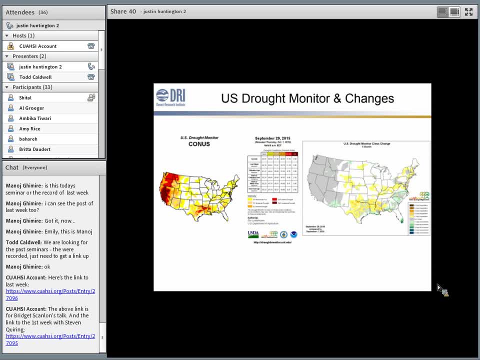 But from the MODIS maps that I showed earlier of NDVI, very large changes, And so I just wanted to point out that using remote sensing, and specifically place-based remote sensing, where you can actually zoom in, Pull out time series, look at specific counties and even farms, is really powerful and really 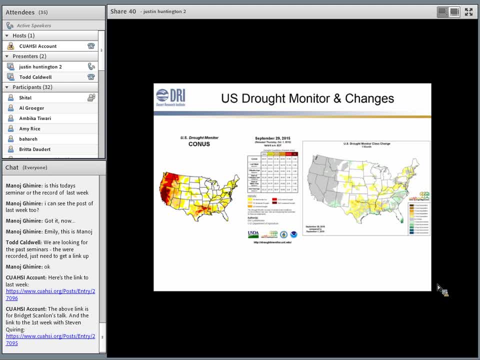 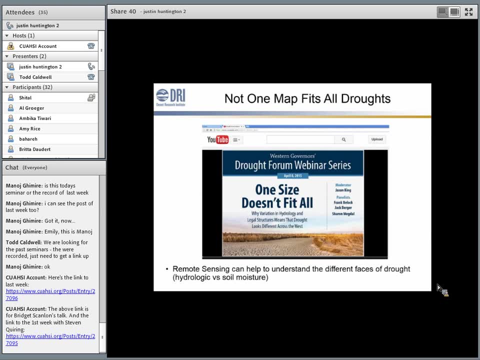 can complement the US Drought Monitor. different classes that are shown. So the point is: is that not one map fits all droughts? And this is a Western Governors Association slide that I took from a webinar series that the state engineer in Nevada, Jason King, did. 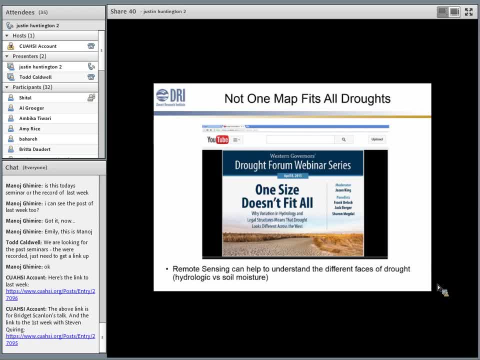 And his point was that, you know, one map doesn't fit all sizes of drought, and that there are reasons why drought looks differently across the West, And it's really tied to variations in hydrology, legal structures and water availability, And so remote sensing can really help understand these what I would call different phases. 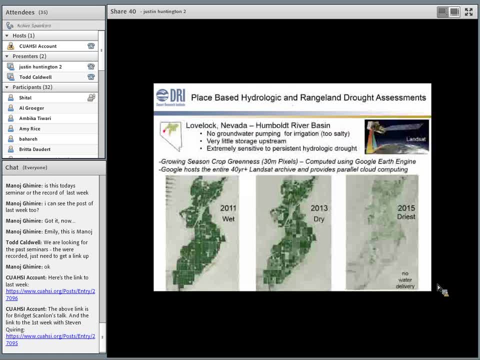 of drought. So here's an example- and I'm going to go through a series of examples- showing how water policy and water sources really makes drought look different in different places. So this is Lovelock, Nevada. It's the Humboldt River Basin. 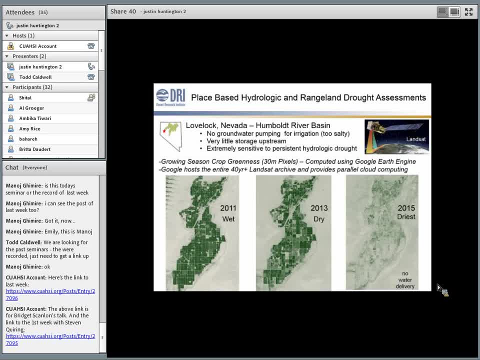 There is no ground for irrigation. Lovelock is in the Humboldt sink So there's very shallow groundwater. It's extremely saline. It's a groundwater discharge area. There's a big ply just to the south So it's a very shallow area. 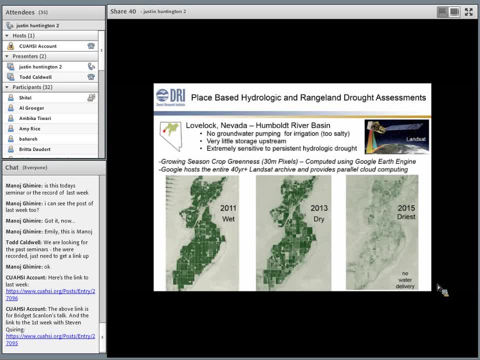 There's very little upstream storage, And so this area is extremely sensitive to hydrologic drought, and especially persistent hydrologic drought. So it's an alfalfa region. Every single field shown here is alfalfa, And so what's shown here is the growing season median NDVI. 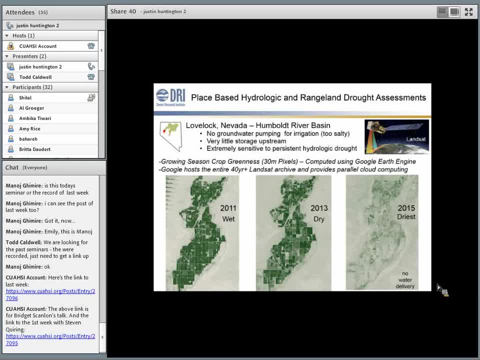 And we used Google Earth Engine to compute this, and Google hosts the entire 40-plus year Landsat archive and provides a parallel cloud computing that I'll be talking about later. But the point is is that you can clearly see how things have dried out. 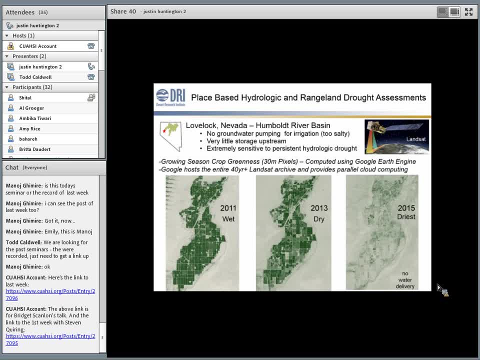 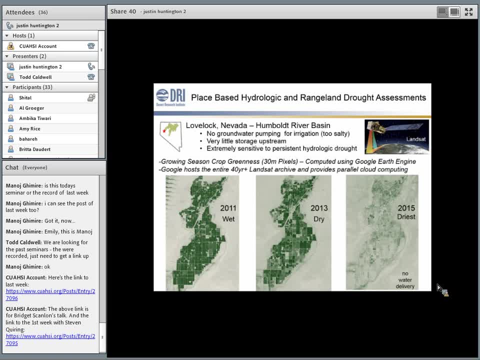 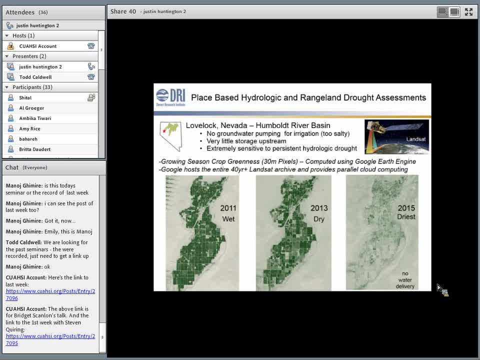 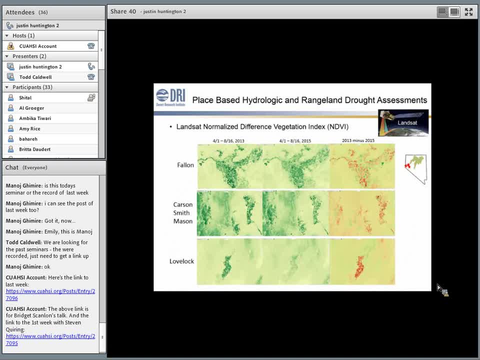 And again I'll show you the trouble, because it sounds like it's based across performance in the tribal communities And obviously the only folks able to do it are sort of the lower enrollment Minnesota communities. But it happens to get unique, like some missions, CC, RWs, the rest are 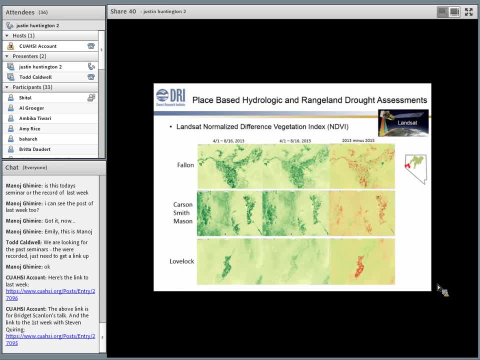 And so if there's something that's missing, it's rather bland- show this water management aspect and impacts of drought that we can clearly see using place-based drought monitoring through. so, Fallon Nevada, here this is the growing season, or April 1 to about mid growing season 2013, and then in the 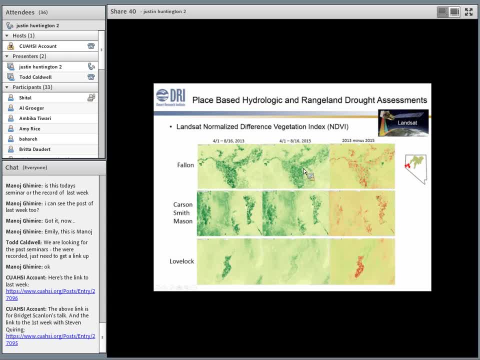 center panel. this is the same date range, but for 2015: median NDVI and all this and then the difference between 2013 and 15. so you can- you can, see a lot of red here, which is means negative, meaning that 2015 had less NDVI than 13. 13 was. 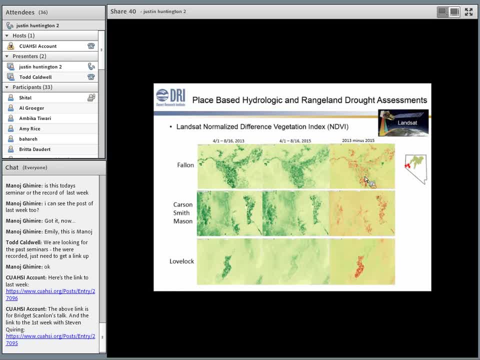 also a dry year, but there was a lot of upstream storage still on the Truckee River system reservoirs. so in 2015, Fallon got a couple irrigations, but very, very limited, and it's why there's a lot of drought in the state of California. 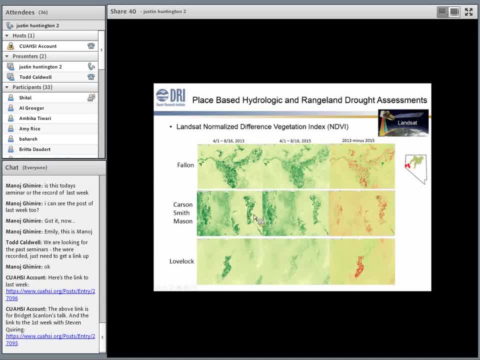 there's a bunch of red. so here's Smith, Carson, Smith and Mason valleys. this is right at the base. Sierra Lake- Tahoe is right over here. Carson Valley: here is very sub irrigated, very shallow groundwater and so you can see that Carson Valley hasn't been that impacted by the current drought. they're high up. 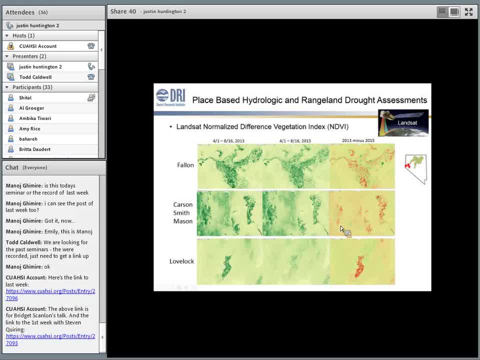 on the river system have more senior rights, whereas Mason Valley it's on the top of the river system and then the river system is on the bottom of the river. different system: it's on the Walker River system. they have supplemental groundwater pumping so when there's no surface water rights available they can. 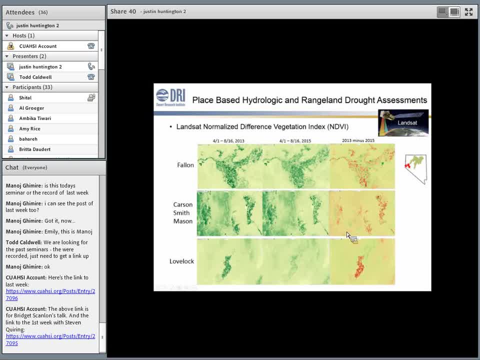 pump, some pump supplemental groundwater and so you can see it hasn't been as impacted as, say, Lovelock, which is shown down in here, down on the bottom, which is a hundred percent surface water driven. so they've been impacted the most. so because of supplemental groundwater pumping in these different areas. 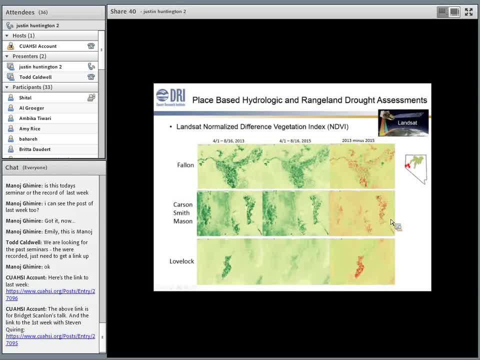 you know, these, these communities are kind of hanging on. that said, their pumping is now impacting the river flow, and so it's it's effect where, because they don't surface water, they're pumping groundwater, which is impacting the surface water, and so now they're pumping even more groundwater because they don't. 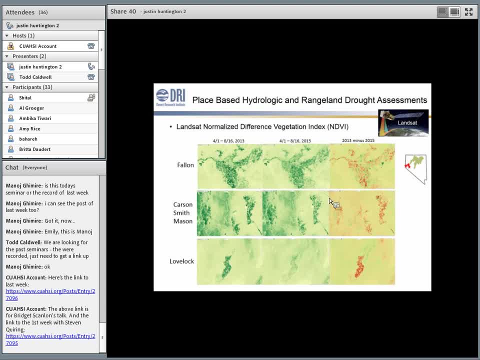 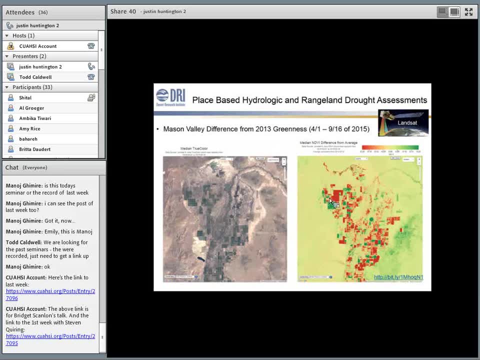 have surface water, so it's a big deal and and we can, we can dig in and look at these impacts. so just some close-ups here. here's in Valley difference from 2013 for this last year there's been some water right buyouts that have happened and and a lot of following going on some 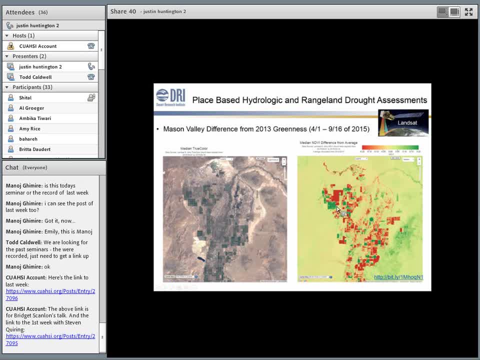 new AG that's gone in. that wasn't her hand in 2013, but the one thing I did want to show is out on the range, here on the desert, you can see this impact of the, the spring and summer rains. where the rangelands are it greener than in 2013. 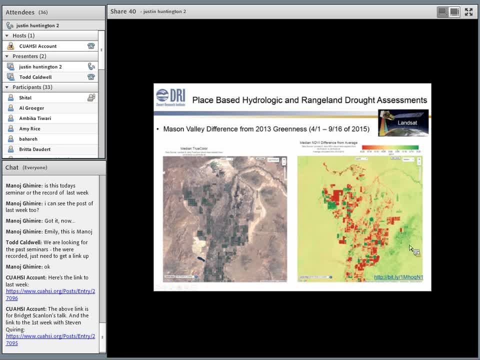 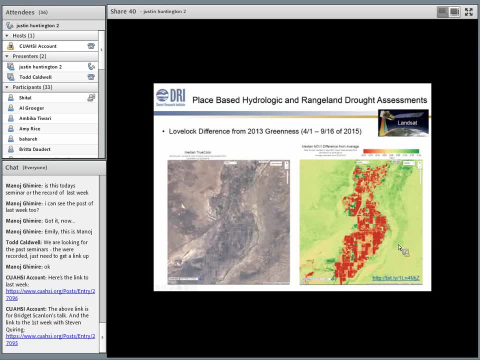 2013,. while at the same time, the irrigated ag has really taken a hit because there's no water in the river. Same thing in Lovelock. So this is a close-up of Lovelock- very, very green out on the range near the ag. 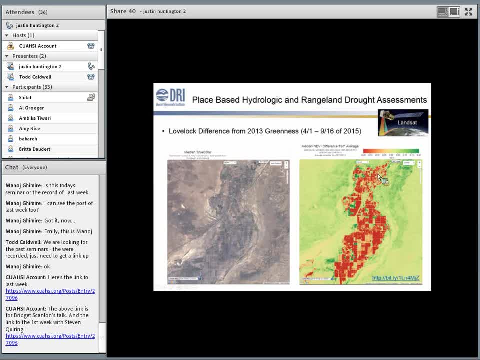 So the ranchers are happy but the irrigators are sad, And it just goes to show how we can have different types of drought happening at the same time in an opposite direction. And normally when you look at these big regional-scale maps or veg-dry-type maps that are generally 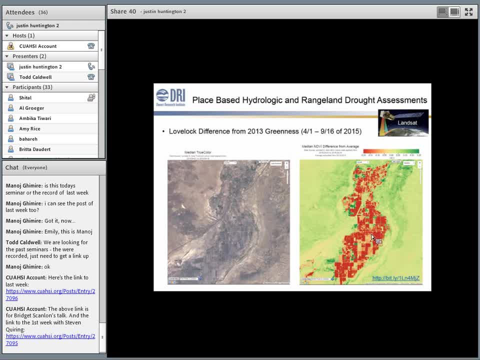 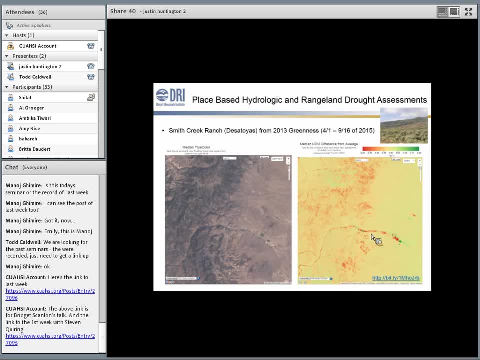 regional in nature you can't zoom in and actually go take a look at this kind of stuff. So just to highlight this point a little bit, more and less focused on ag but more on range. this is in central Nevada in the Desatoy Range, Smith Creek Ranch. 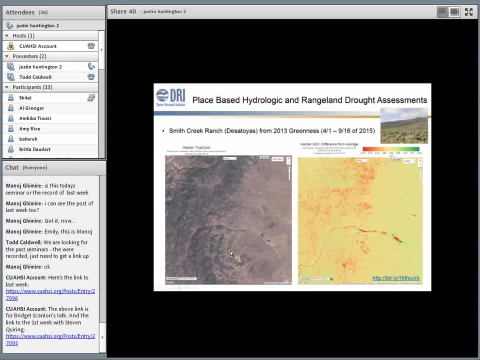 There's a bunch of pinyon juniper out there. They're up in here And you can just see the impact of this year's drought, relative to 2013, on the riparian zone and also the pinyon juniper. So there's been a lot of pinyon juniper die-off this year because of the very, very low snowpack. 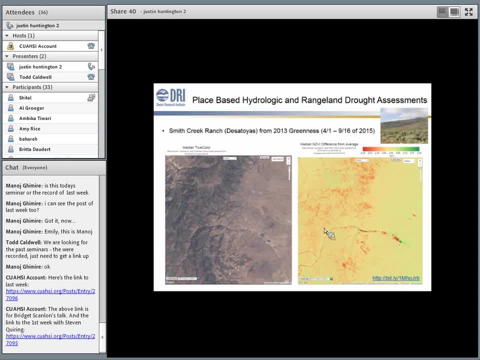 that we've received And now we're basically in the third year, And because PJs have deeper roots, of course, in the grasses, they're more susceptible to this hydrologic-type drought And it didn't really respond to the drought. 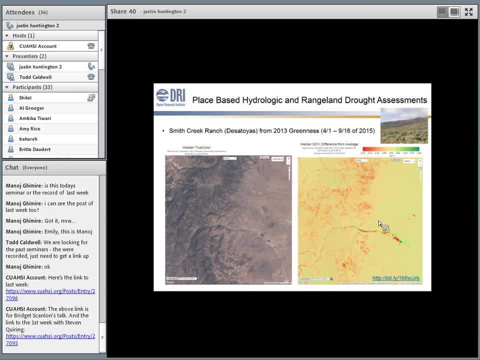 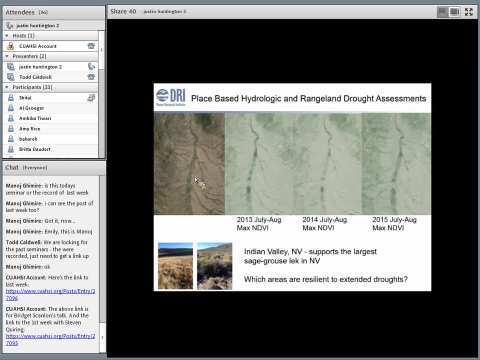 It didn't really respond to the spring and summer rains that we had, because that basically just got all evaporated and transpired, And so the PJs are still pretty stressed. Here's a series of riparian zones. This is called Indian Valley, Nevada. 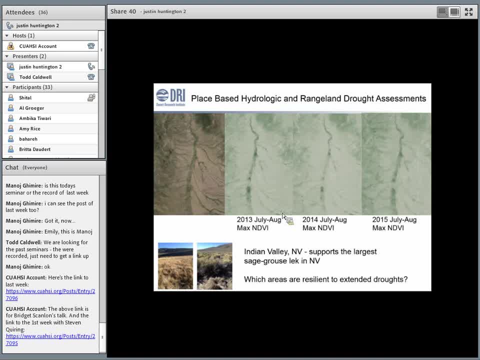 This has got the highestthis valley supports the largest sage-grouse lek in Nevada. Basically, the populations of sage-grouse here are higher. They're higher than the average. They're higher than the average, So they're higher than the average. 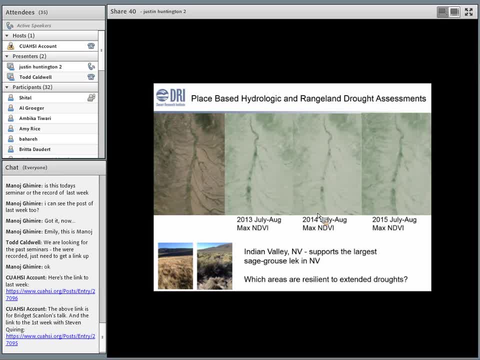 They're higher than the average, So the biggest in the state. And so the BLM wants to know, when creating sage-grouse for FUSA, which areas in this valley are most resilient to extended droughts. If we're going to put up fence and protect certain areas, where do we protect? 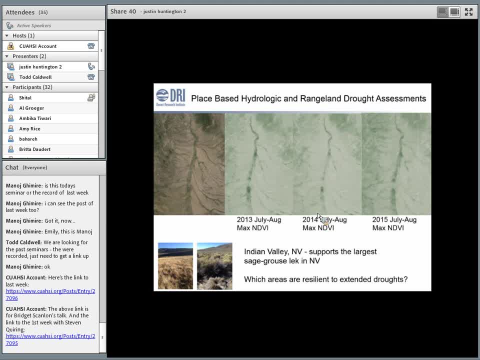 And we want to try to identify where the vegetation is persistent even through these long periods of drought, And so you can potentially identify where the vegetation is persistent, And so you can potentially identify where the vegetation is persistent, And so you can potentially identify where the vegetation is persistent. 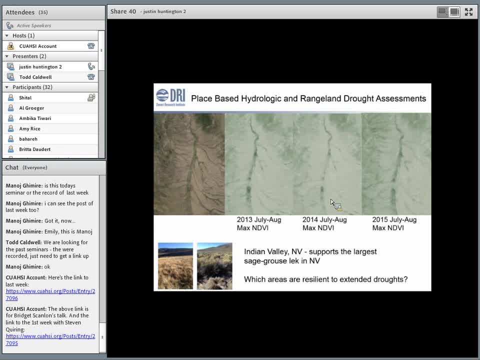 And then we can also identify areas such as here, And you can see how 2015 was quite a bit greener than these other years because of this relatively wet spring and summer that we've had. But we can finally dig in and identify some of these things with Landsat-based remote. 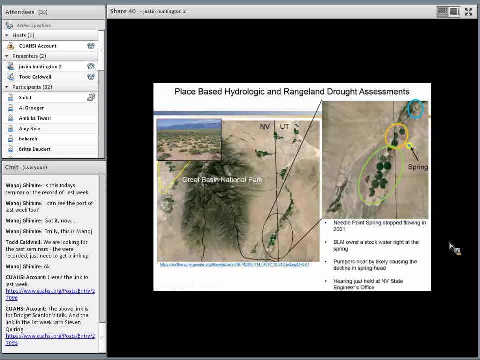 sensing And then just to further dig in to impacts assessments and using Landsat- there's a little bit of a mix there- to look at drought and and other things like water management and try to separate out the impacts of water management from drought, which is not always easy to do. this is needlepoint spring. it's near. 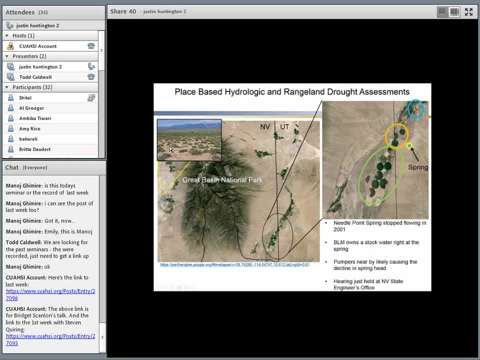 great basin national park, which is right here. there's several down in the southern portion of snake valley. this is right on the nevada- utah border. this happens to be the area where southern nevada water authority has applications to pump groundwater and ship that water to las vegas, and 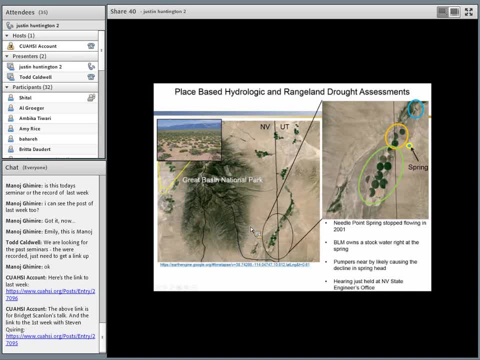 so this is a very contentious area and this spring, called needlepoint spring, went dry in 2001.. the blm owns a stock water right to this spring and the pumpers nearby likely caused the decline in the spring. head here and this is a water rights hearing. that's that they got held in the room. 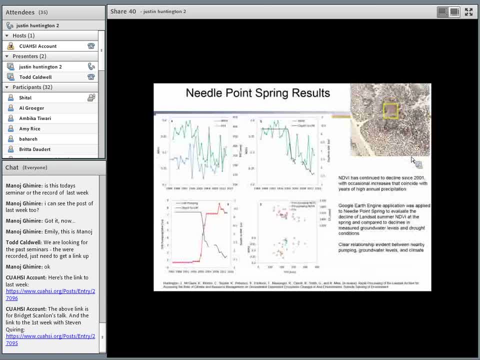 has yet to be written, but basically what we did was compare our vegetation index time series shown here. this is derived from Landsat Landsat 5,, 7, and 8, where we did a spatial average over the spring area to look at NDVI over time and you can see that right around. 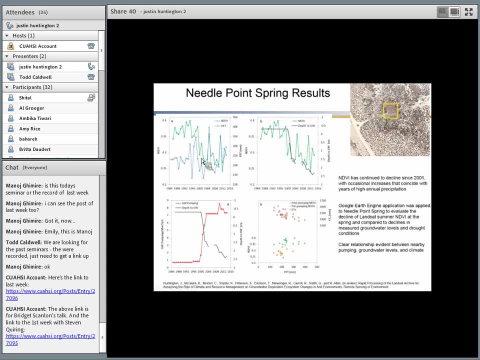 in 2001,. the NDVI dropped dramatically. What's shown here is precipitation. This is water year precipitation and you can see that the NDVI generally tracks precipitation, except for this big drop, which also, I should say, tracks precipitation. That's part of the problem. 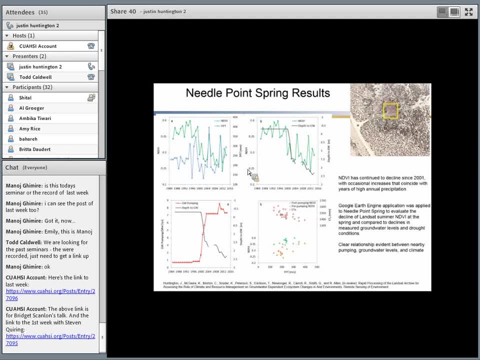 here is that there's a big drought that started in around 2001,. so is it the pumpers that caused the decline or is it the water, The drought? So we did an analysis where we looked at the pumping. the pumping ramped. 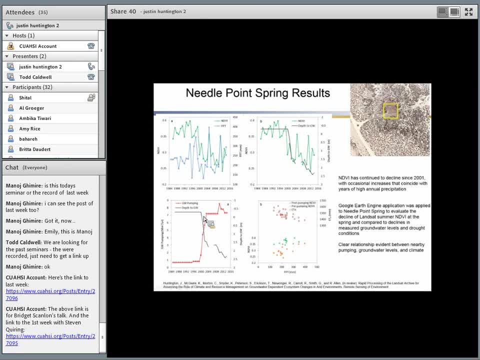 up the head at the spring declined as soon as the pumping ramped up, and so if you plot NDVI with the depth of groundwater at the spring, you can clearly see there's good correspondence. and of course there's some big spikes in here when we have big water years. but the bottom 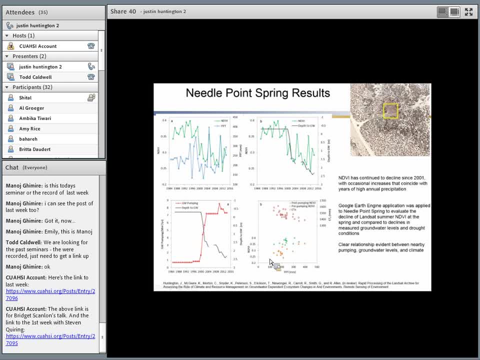 line is that when we start to look at things, what we're seeing is that there's a lot of heat flux. We call it a complementary space, where there's a complementary relationship, basically between reference evapotranspiration or Pema-Monteith and ET, or using NDVI as 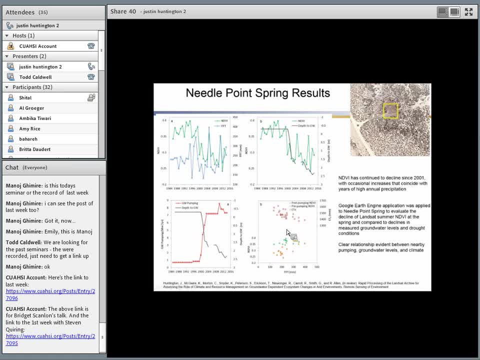 a proxy to ET. Generally, when ET goes up, reference ET goes down because of that feedback effect. When ET increases, we have more humidity in the air, less sensible heat flux, and so we're seeing that there's a lot of heat flux. 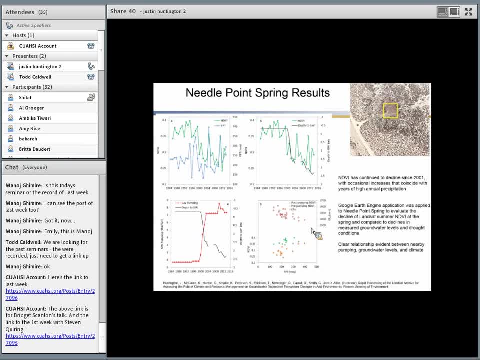 Thank you, Because you have a higher latent heat flux. typically, when we have higher precipitation, you have lower solar radiation because there's more clouds, more precipitation and higher humidity, and so this is called the complementary relationship. So what we did was just plot. 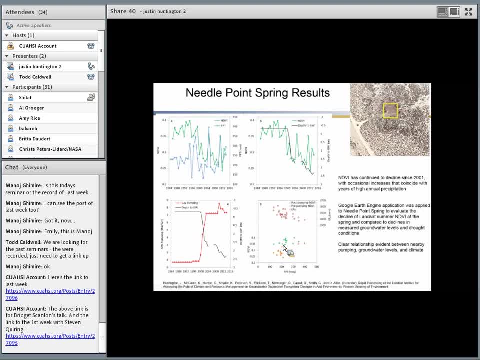 post-pumping and pre-pumping and so for the same given amount of precipitation, you have much lower NDVI. USGS has modeled groundwater. We're looking at much more groundwater levels in this area and the impacts of the pumpers, and it's pretty clear that the pumpers cause this spring to go dry, The point I'm trying 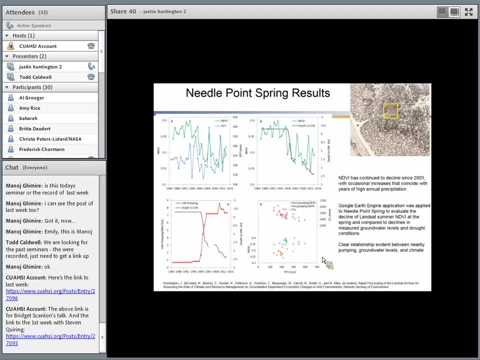 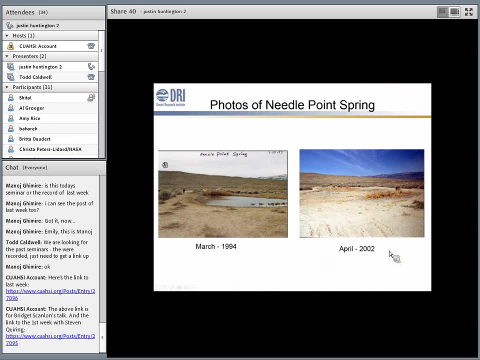 to make is that, using remote sensing and paired with climate information, we can start to tease out the impacts of drought versus management. These are just some photos of the Needlepoint Spring area. This is all grease wood and salt grass out here. So friata fights shallow groundwater, sandpit, lands, storey sandpit. and many, many other depths out here, And then you can see here the troubles with the water. This is all in the middle. It's very high, very low, but it's a little bit of a walk rate. I'll just ask the panel if you could show me where this is just showing you. 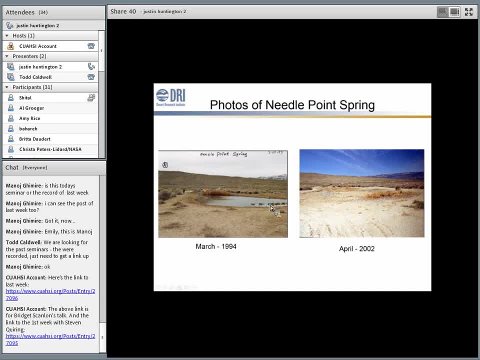 roots are tapped into the capillary fringe and the phreatic surface of the water table. This is what it looked like in 94, and then this is what it looked like after the pumping started in 2001 and the spring went dry, although there was also a drought going on. 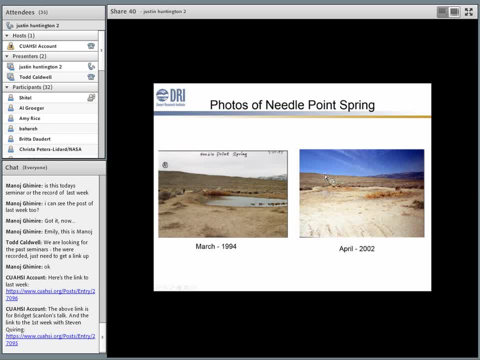 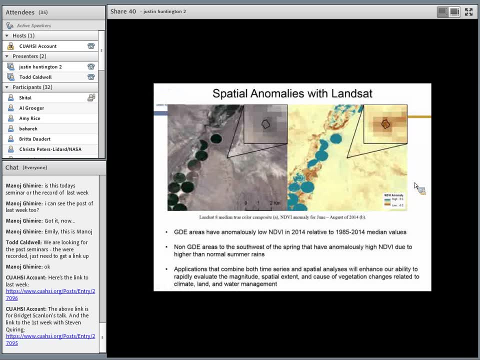 But in general, you know, it's like: well, how far in space is this impact extending? So that's where we went. next is creating spatial anomalies with Landsat to see kind of what this looks like in space. So this is the NDVI anomaly through August of 2014 relative to the full Landsat climatology. 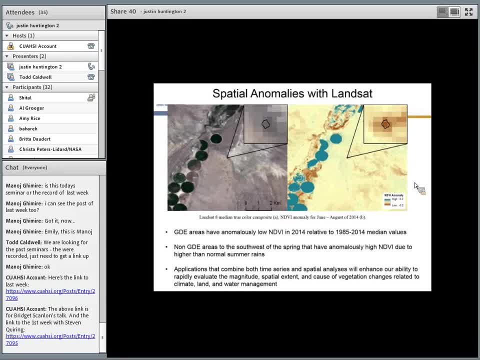 from 1985 to 2014.. Now, to do this locally on my box, my PC here, you know, I'd have to have the whole Landsat archive, of course, And write a bunch of scripts to make these anomalies, and it's just, it takes a lot of. 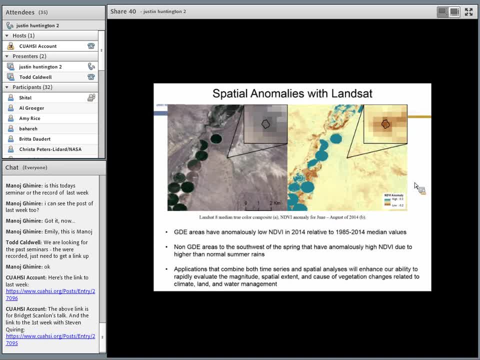 time and storage and computing power to do that, And so we used Google Earth Engine to do this, and it really is changing the way we do things, And being able to combine time in the spatial analyses is really greatly enhancing our ability to rapidly evaluate the magnitude and spatial equation. 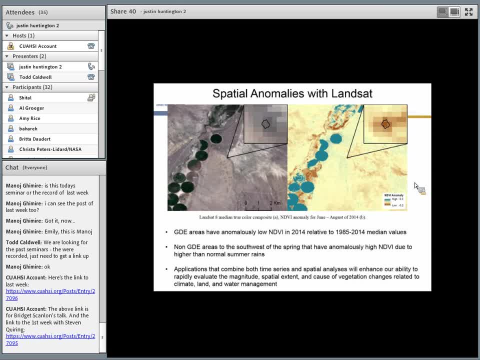 So it's a big tool that's coming out of that And so you know it's a very, very, very important tool to go forward. So we're going to have to try and build on that as well. So I'm going to go ahead and put this slide up here. 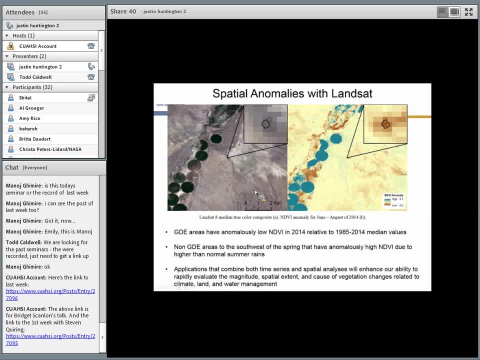 And it's a little bit of a game changer in terms of how you can get this and how you can get it to work. So what we've found is that, you know, this is a very, very interesting activity, And what we're going to be looking at is the way we're going to be working on it. 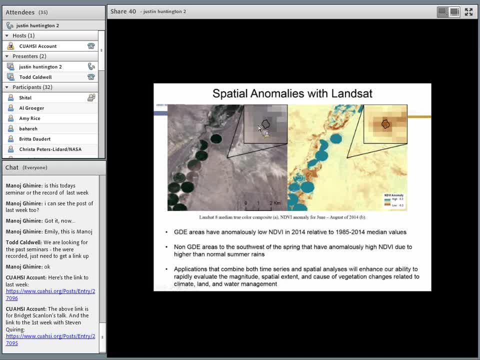 And so you know we'll talk about the future of this. you know some of the things that we've been working on for the past two years, But what we're going to be looking at is where the future of this is going to be, and then what we're going to be looking at is how we're 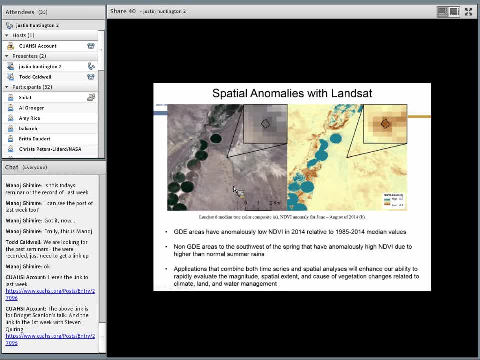 sagebrush rabbit. brush Over. here you can see the impact of the recent summer rains. We had an anomalously green vegetation, whereas in the phreatified areas, where the vegetation is living off the shallow groundwater, we have an anomalously low NDVI, even though 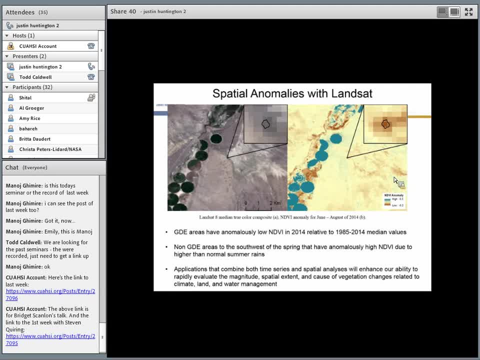 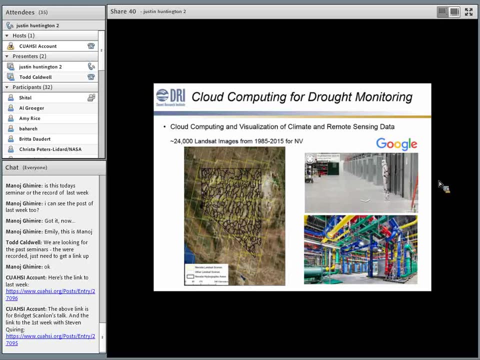 it was a fairly wet spring and summer. The groundwater levels have dropped and have affected the groundwater-dependent ecosystems in these areas. To this cloud computing stuff. just to kind of recap on just what was required to do this type of work where you look at Landsat scale anomalies. basically, if I wanted to do this, 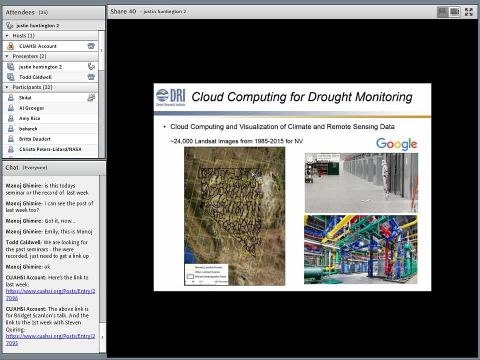 for the whole state. I need 24,000 images. That's the collection that exists for between Landsat 5, 7, and 8.. We just can't handle that. We are relying on Google, who has ingested the full archive. 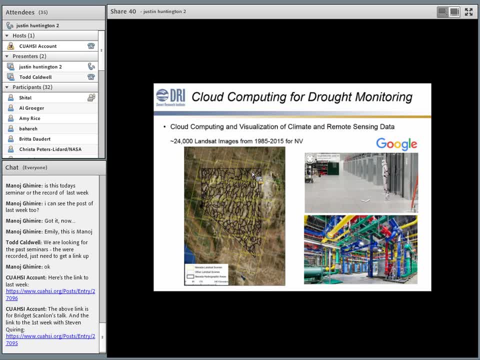 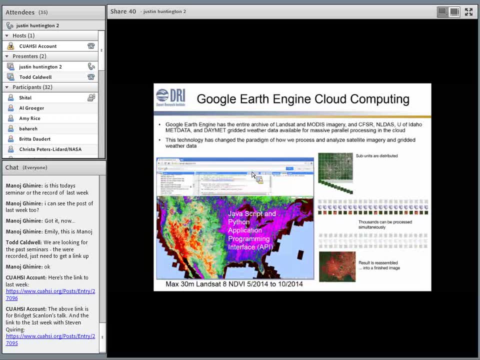 of Landsat, as well as MODIS, and utilizing their cloud computing system, As I mentioned, Google Earth Engine. they have the entire archive of Landsat and MODIS, as well as a bunch of different climate datasets that they've relied on us to help them know. 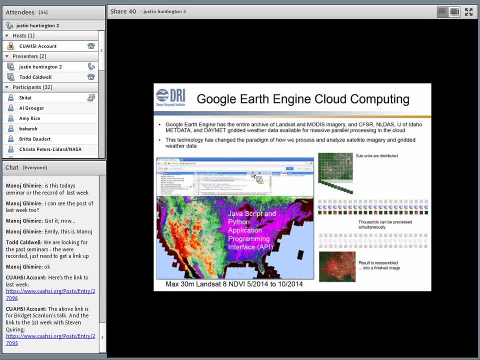 about and ingest into their systems. We have the Climate Forecast System Reanalysis. We have NLDAS, the North American Land Data Simulation System, and then this bias-corrected and downscaled NLDAS dataset called the U of I MET dataset by John Abbotsoglou's group, as well as DayMET. 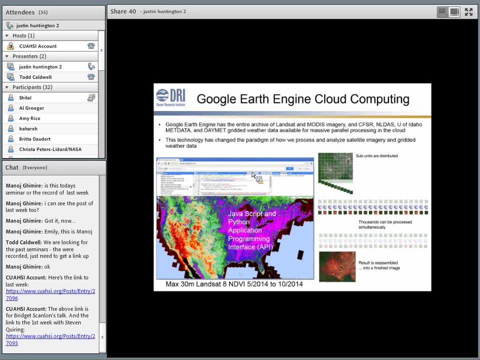 Now, I just loaded up GL version 1 and 2.. All this is in the cloud and available for everyone to access, And so, basically, what Earth Engine does is they break out these image collections, they call them into lots of different units and they parse out those units into thousands. 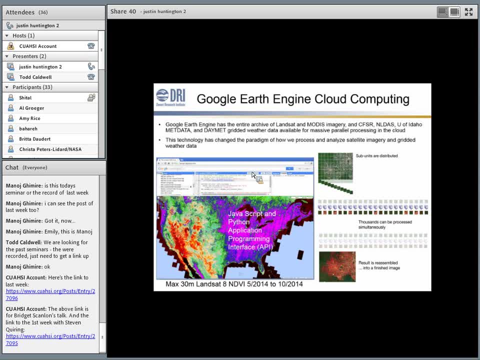 of different computers to process those units all simultaneously and then stitches everything back together, And so there's a Python API app programming interface as well as a JavaScript script application interface, And the JavaScript API is called the Playground, and it's really great. 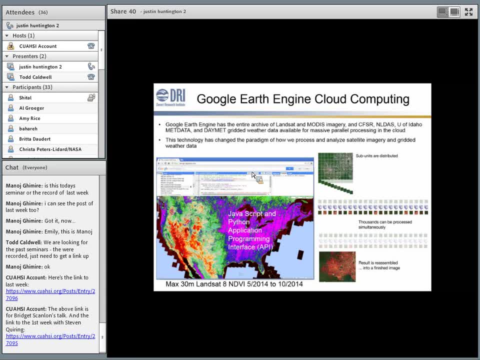 You can just write JavaScript code, call in image collections, make simple computations and it makes a map immediately. So this Landsat scale map, Landsat 8, NDVI, for basically the growing season of 2014,. basically took about 15 seconds to create 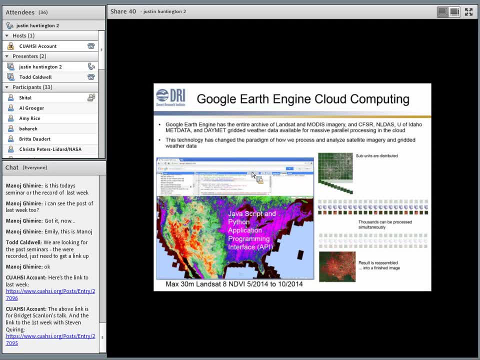 Now, Google Earth is a little bit more advanced. Google Earth is a little bit more advanced. Google Earth is a little bit more advanced. Google Earth Engine doesn't actually process every single 30-meter pixel at a scale like this. It groups pixels together to a scale that is meaningful at this scale. 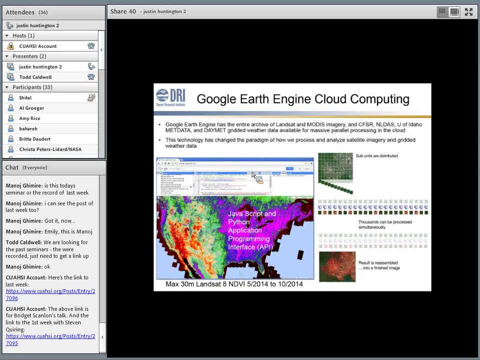 You don't need to have 30-meter scale to get information out that's meaningful at this scale. So they aggregate to larger pixels and then do the computations. but as you zoom in it resends those calls And then it will do the computations at finer scales. 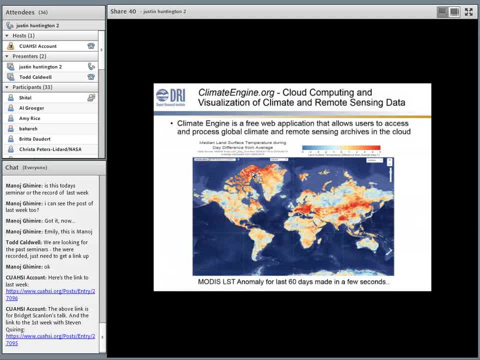 So on to climateengineorg. what is this? It's basically a cloud computing and visualization of climate remote sensing data. It's a free application that allows users to access and process global climate remote sensing archives in the cloud. So this is a MODIS land surface temperature anomaly for the last 60 days. 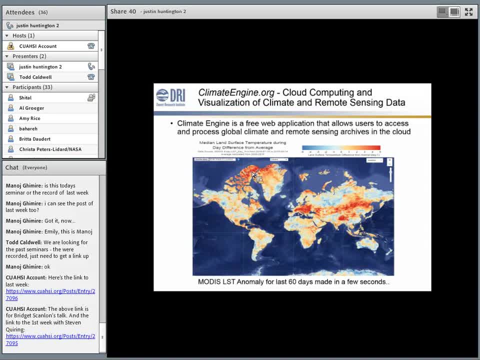 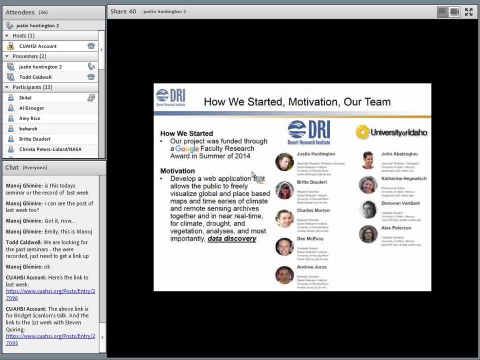 I'll show you this in a few seconds, And that's really the first page of our web application. So imagine trying to make this locally at your institution. It would just be a nightmare. So very, very neat developments. How did this get started? 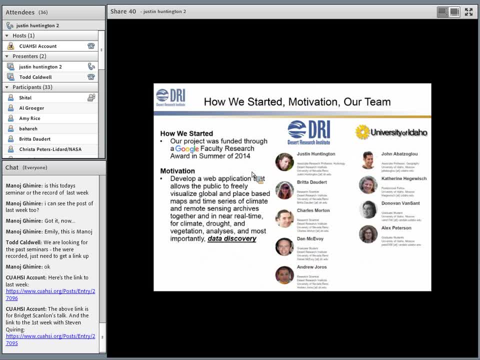 Basically, we applied for a Google Faculty Research award grant and we were awarded to start a drought monitoring program in Google Earth Earth Engine, and from drought it turned quickly into climate and remote sensing, And so it's a web application that allows the public to freely access and visualize. 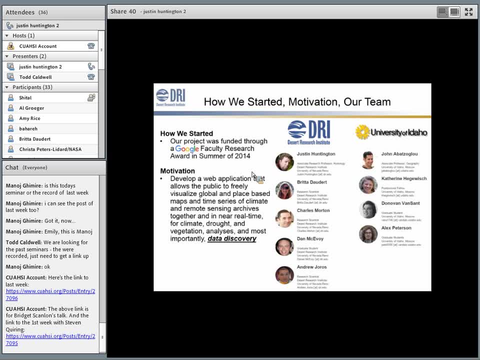 all these things- maps and time series and in near real time for drought, vegetation analyses and, most importantly, data discovery. And I have emphasis on data discovery because, you know, in the past we just haven't been able to explore what the data have to offer. 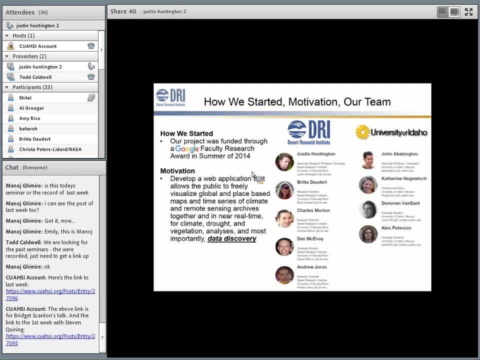 And now we can see all these neat things. It's just really opening the door into all different types of things that we've really never been able to think about because we couldn't visualize it. So I'd just like to really emphasize that this is really changing how we think about. 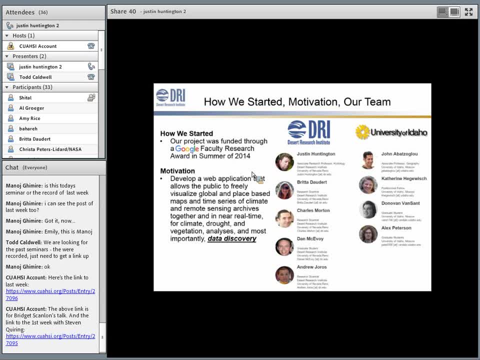 things We conduct research by being able to see things and then generate hypotheses, instead of thinking about hypotheses and then trying to visualize what we're thinking about. It's really changing the way we do things. So it's a very collaboration between DRI and University of Idaho, between John's group. 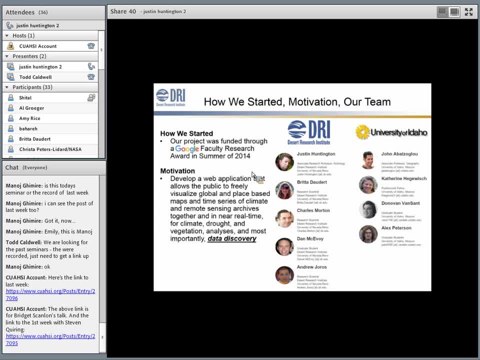 and our group, And I'd like to really Give hats off to Britta and Catherine at University of Idaho and Britta here at DRI, and Charles Morton and Dan McEvoy and Donnie and Alex and Andrew, who are really the folks that have made this happen, especially Britta and Catherine. 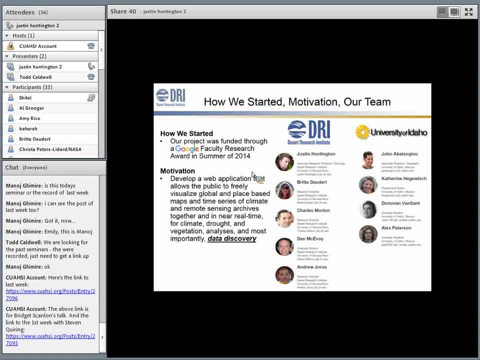 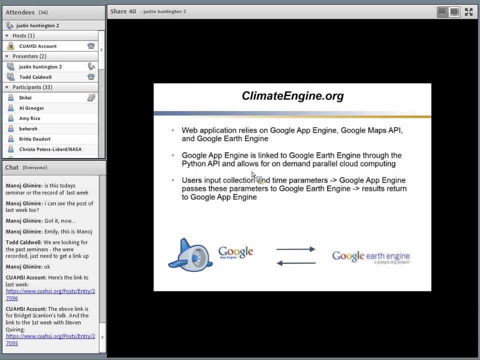 They've poured their hearts and souls into making this web application and work on it basically every day. So this thing Web application relies on. It relies on Google App Engine, which is basically the front end, and Google Maps API, and then Google Earth Engine is the back end. 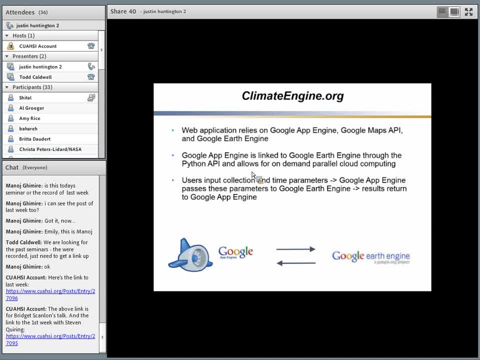 And so Google App Engine is linked to Earth Engine through the Python API and allows for on-demand parallel cloud computing, And so basically, users input collection and time parameters through the Google App Engine, and then App Engine passes these parameters to Earth Engine in the back end and then 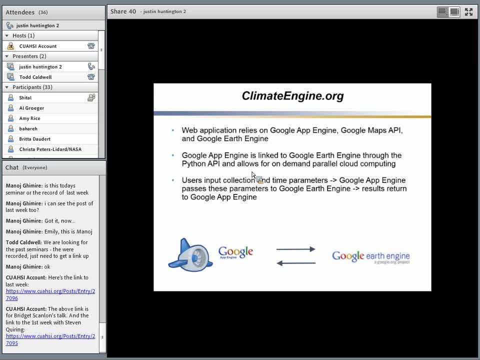 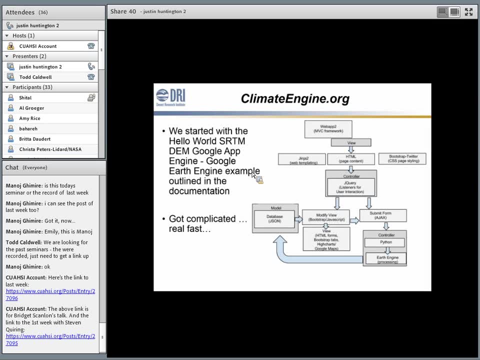 the results come back into the front end or Google App Engine. Okay, So So we started out with the Hello World SRT MDM App Engine example, and anybody can sign up for Google Earth Engine and there's a developer's forum and if you want to make 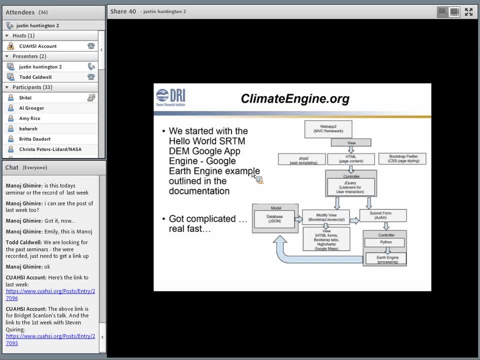 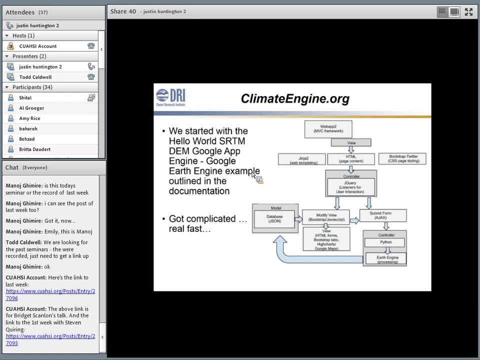 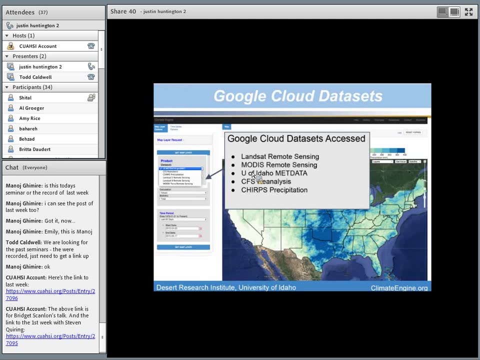 We kind of took it to the next step fast, and it got complicated really fast. We aren't professional web dev folks, and so it was definitely a big challenge for us, but we managed to plow through it and have made this application called Climate Engine. 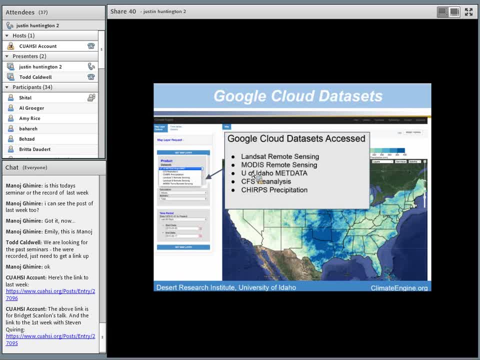 which I'll go through next. So So we basically have a collection of different data sets available to access and process: Landsat MODIS, this U of I MET data, CFSR, and then Chirps, Precipitation, which is a. 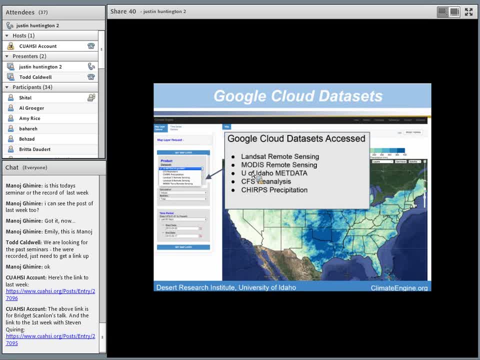 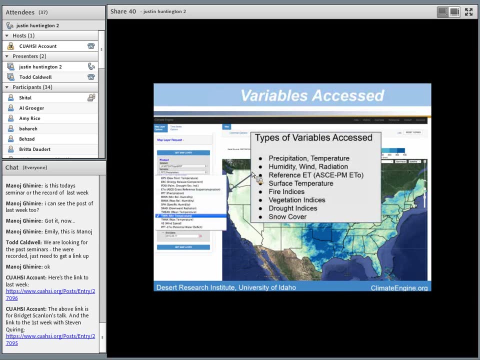 global precipitation product, a Pentad or five-day time scale, and I believe it's 19 kilometer resolution. So you can access these different data sets and once you pick a data set, then there's a whole host of different variables within the data set. 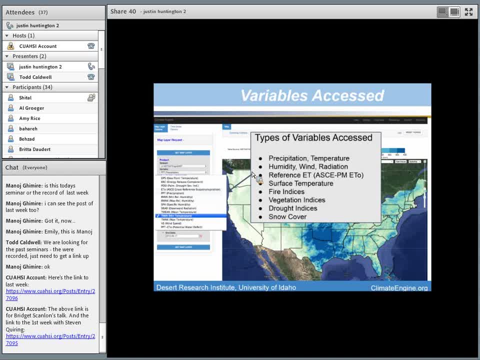 So we have precip temp, humidity, radiation, We have Pememonti- they're physically based reference ET, PDSI also with physically based reference ET used as the potential ET in PDSI of the typical Thornthwaite equation fire. 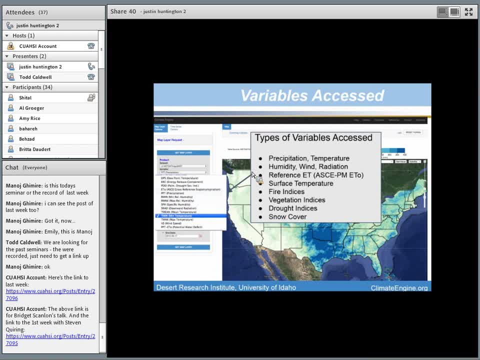 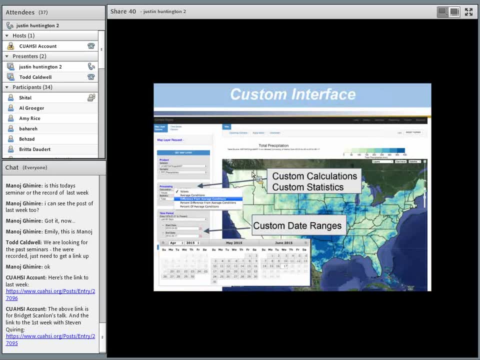 indices, veg indices, drought indices, snow cover, lots of different things depending on the different data set you pick. So Custom statistics, so average difference from average percent, difference from average percent of average, and then we even have percent in the distribution. 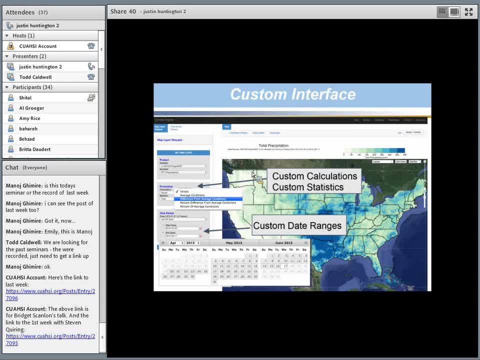 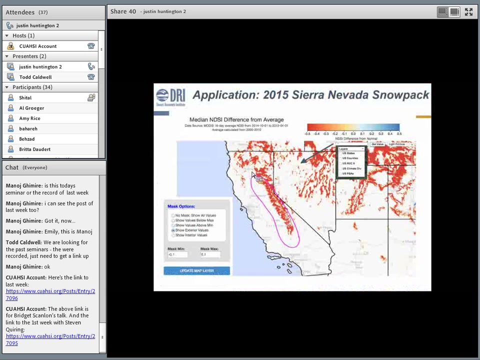 And we're working on different non-parametric ways to depict drought and anomalies rather than using parametric distributions- things like SPEI with gamma distributions and things like that, So you can pick custom date ranges, And so here's just some applications that I'm going to run through. 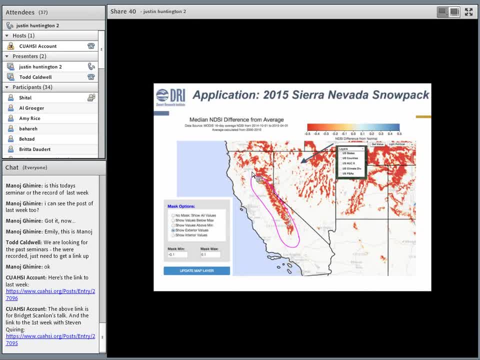 So here's the 2015 Sierra Nevada snowpack median normalized difference. snow index difference from average for basically October through April, or to April. for this last year, Everywhere in red should have been covered in snow and it wasn't this last year. 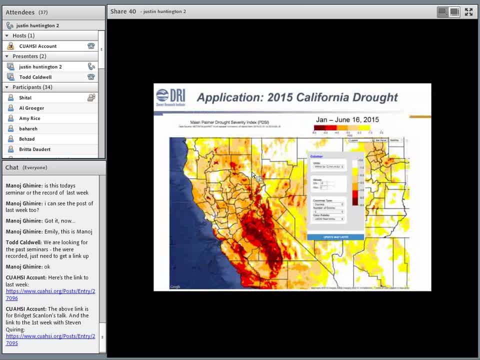 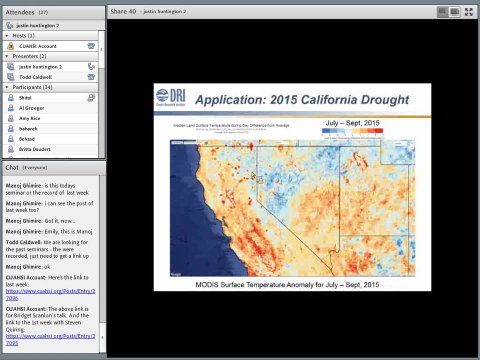 Pretty dire. Here's PDSI. Here's the snow. This is January through June of 2016.. We have the USDM drought color ramp in here to make maps more visually comparative to the USDM map. Here's median land surface temperature difference from average for July through September. 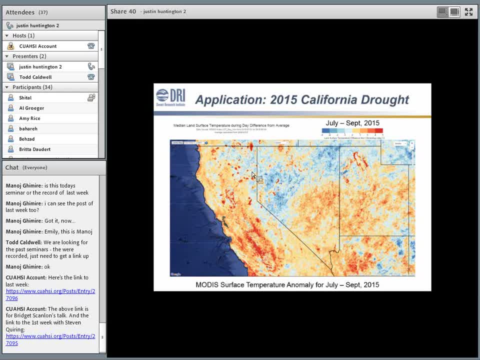 I really like to look at this land surface temperature anomaly type product because it gives you such a good sense of the land surface energy balance and evaporation. So, And you can see, here is a lot of evapotranspiration. Where you have cooler surface temperatures, you typically have higher evapotranspiration. 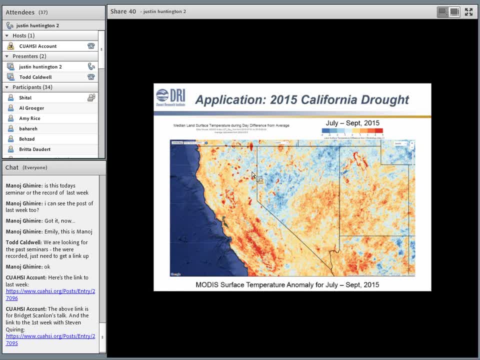 becauseand that higher evapotranspiration in turn creates evaporative cooling and therefore surface temperature. So it really does tell a nice picture of latent heat flux. In fact, most land surface energy balance models that compute ET, most of them, are latent. 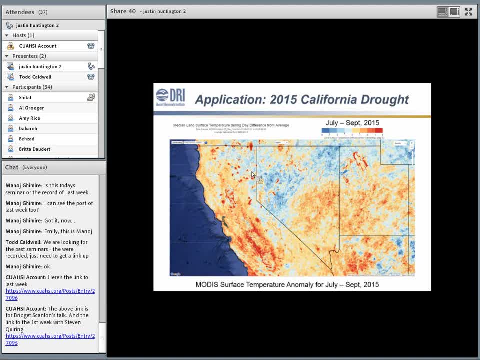 and most of them are not. And you can see, here is a lot of evapotranspiration. So you can see, here is a lot of evapotranspiration, largely driven by surface temperature, and the relationship with surface temperature and P is extremely strong. 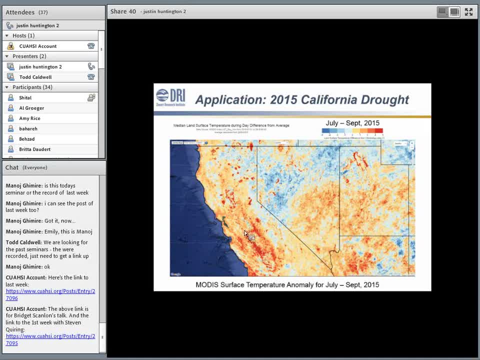 So what you can see here is that this abnormally wet summer, ie high evapotransmission summer, but then embedded in here are all these little irrigated areas that I showed you before. Here's Lovelock, abnormally hot because there's no ET happening. same with Mason and Smith. 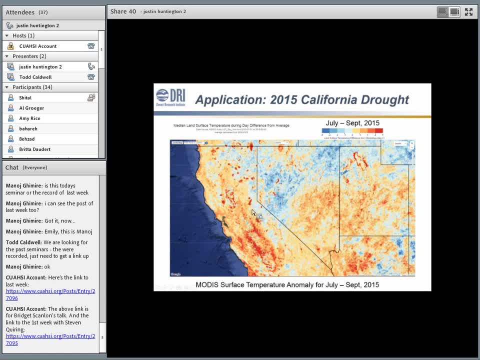 Valleys and then you can see a bunch of fire scars. This is the big fire that happened in Yosemite last year. the year before This is a big fire that happened near Pollock Pines, So really neat. You can see the decline in the Salt Lake. you can see the shoreline that should be covered. 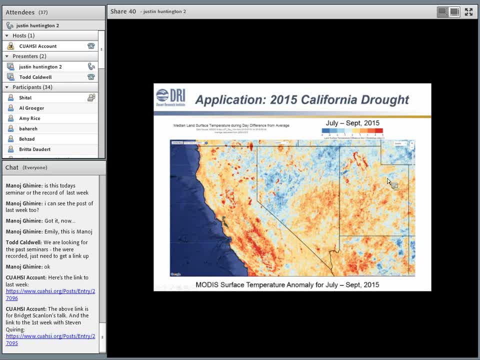 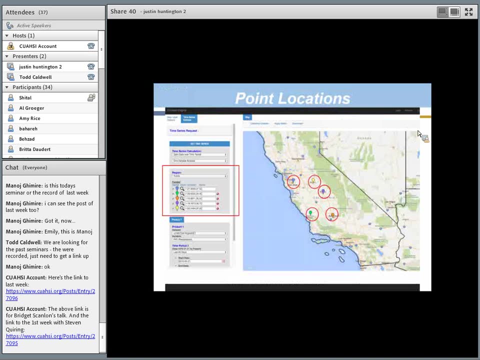 with water and it's not So really intriguing things that you can see. Of course, the Central Valley is all dry because of the drought, So land surface temperature tells you so much about drought conditions And land surface energy balance feedbacks. So point locations, you can pull out time series for different points and then be able 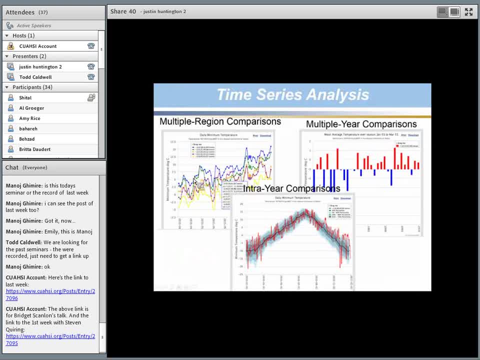 to plot those points together for inter-comparison. You can plot the daily time series of MODIS and DVI or any climate product that we have. It's all the same functions for plotting, You just pick different data sets, basically Intra-year comparisons. 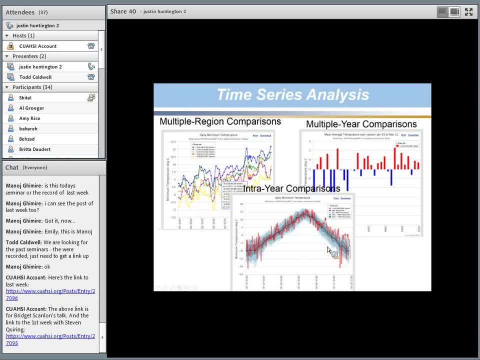 So you can look at within-year variability relative to the long-term and then multiple-year comparisons. So you can start to say: hey, I just want to look at June through September for every year, going back to 1985, to look at summertime effects for every year. 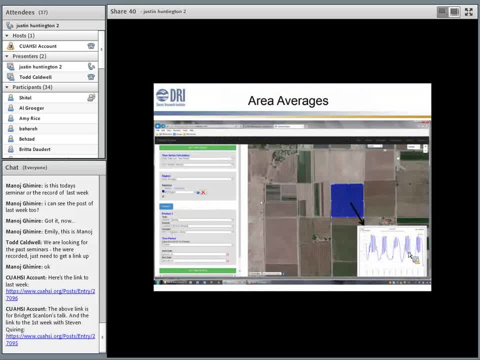 So that's kind of nice. And then you can also draw polygons around, say, for example, a specific field, and then pull out the NDVI time series. So that's really neat. It's a spatially-averaged time series for a field. 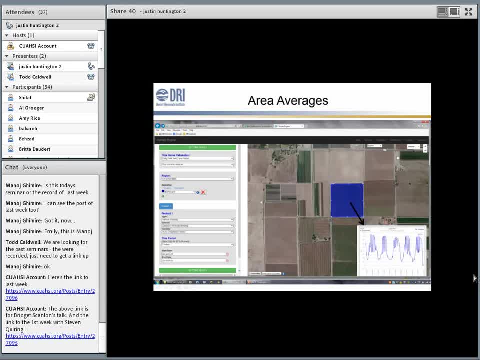 And so what's shown here is an alfalfa field and you can see the cuttings of alfalfa. Here are these spikes, These are cuttings. This is in Mason Valley, Nevada, But basically these guys aren't being impacted by the drought because they're pumping groundwater. 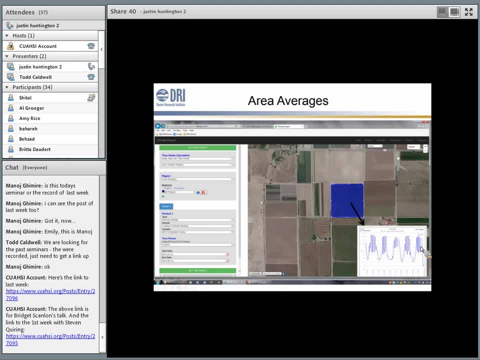 If I were to make a polygon in Lovelock, you'd see the cuttings and then for the last two years it'd basically be a flat line. So we can do field-scale monitoring, Field-scale monitoring of vegetation, which is really new. 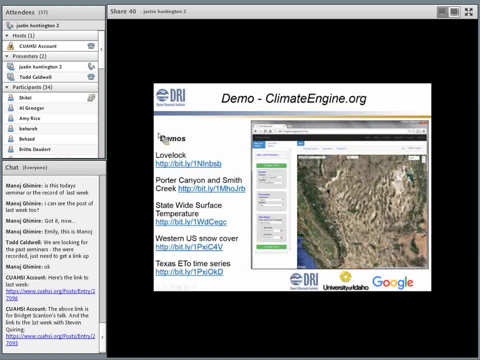 So I'm going to do a couple of demos now and give it a shot, see how it goes. So this is: what's really neat is you can click on link here Once you've made the map, you can click on the link, this link button, and it'll give. 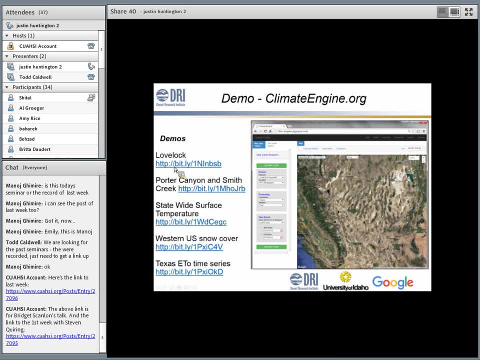 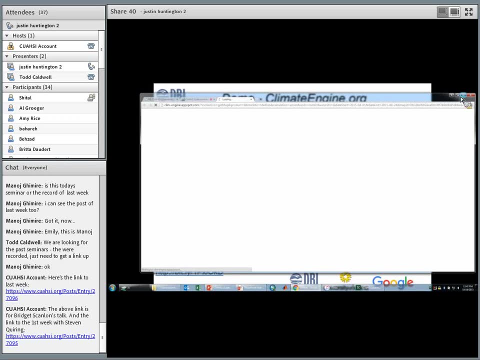 you a link that then will basically embed all the map parameters, the web parameters, into the URL And we'll then- Okay, We'll then go create the map for you in real-time in the cloud. So let's see how this goes here. 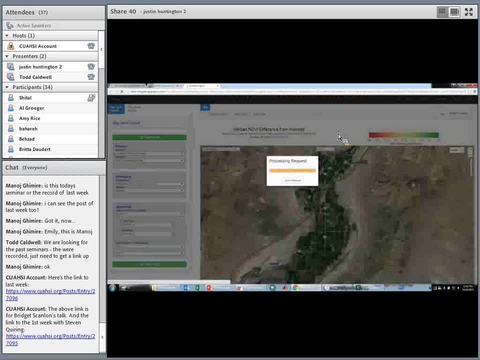 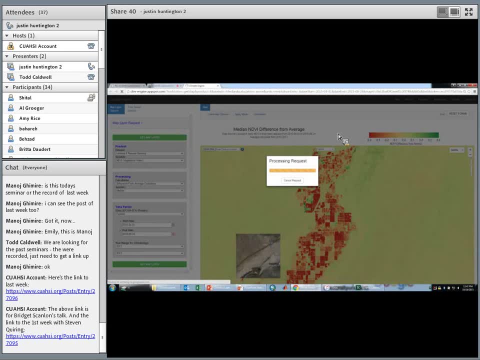 It's All right, So it is making the map right now. Now, I clicked on the link earlier and so this results in the cache. That's why it's coming up so fast, These little squares that you're seeing. these are all results coming back from different. 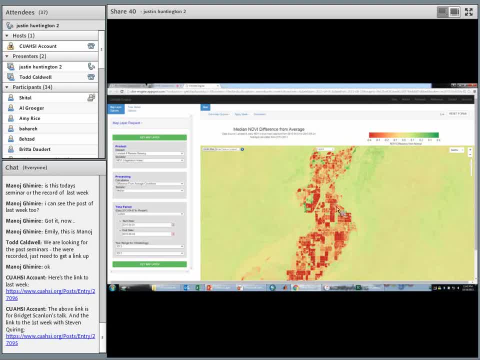 computers at Google, But you can see the clear and the dry. You can see the change conditions. Now I'm going to go to the north here a little bit and go upstream where there's groundwater pumpers. Now Wright Patch Reservoir is all green because there's no water in it and there's a bunch. 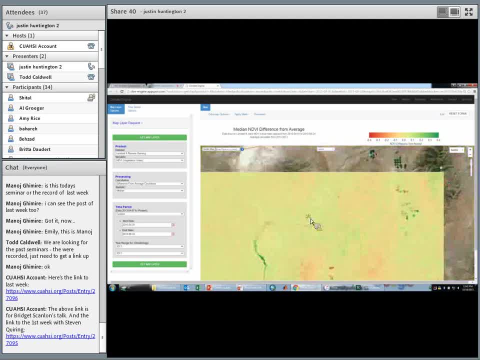 of weeds growing in there now, But let's keep going upstream here and we'll see all these center pivots that really aren't that red. So this is a big pumping area next to the Humboldt River called Winnemucca Farms. 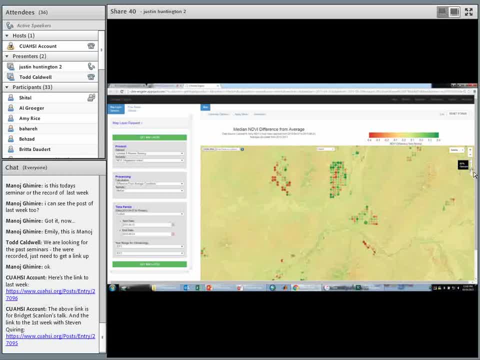 And this is Okay. So this is because the water is getting very, very wet. So a lot of these fields have been pumping and most of their fields are abnormally green, because we've had kind of a wet summer and the evaporative demand's been fairly low. 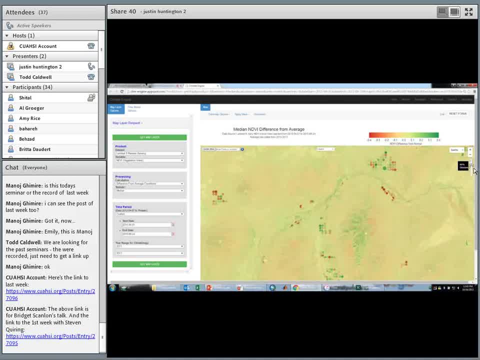 and so those crops are doing really well and they're just pumping. So you can start to get a sense for who's being impacted by the drought and who's not. And the more you scroll around, the more calls go out to the Google Cloud. 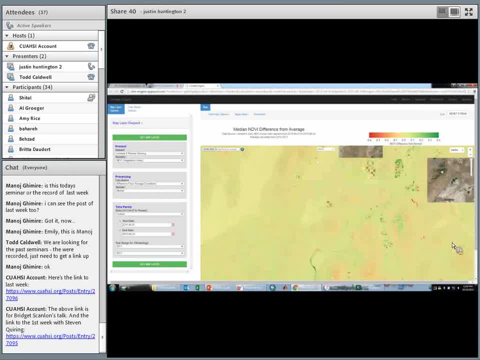 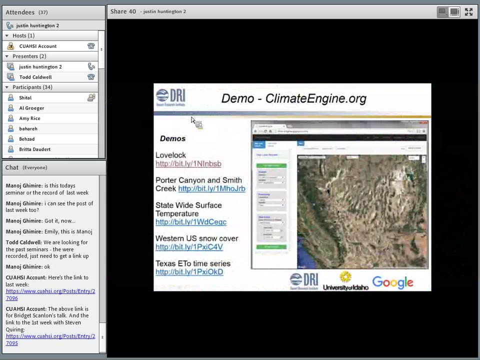 calls go out to the Google Cloud and we'll keep on doing the computations and pulling data. So pretty powerful stuff. Let's go back to my talk here and resume slideshow. Yeah, let's go to this western snow cover. I showed that earlier, but I want to show it again in. 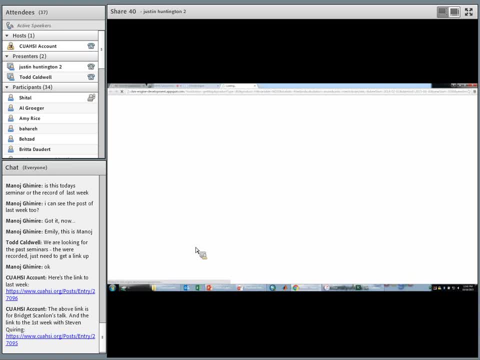 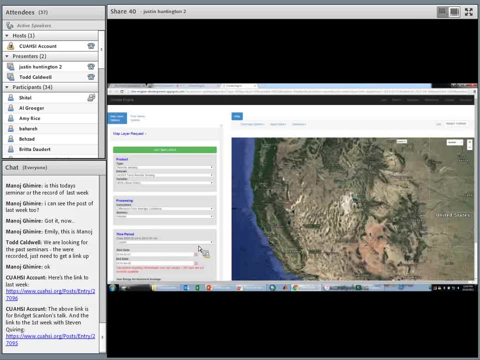 more of a live version. All right, so it's making the computations. now It should be coming up. Okay, Git map- Uh-oh, not working, All right. well, I'm going to go to these examples. So we have some examples on the. 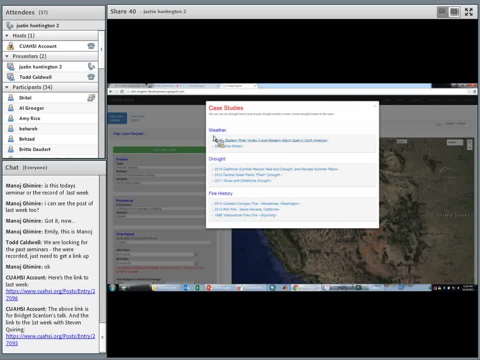 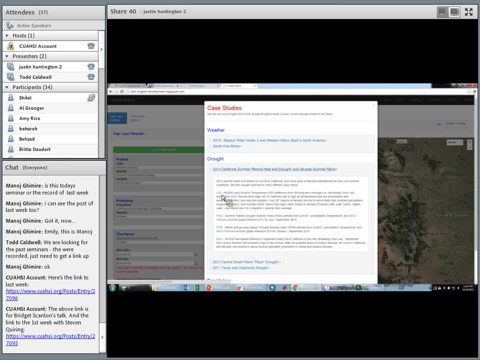 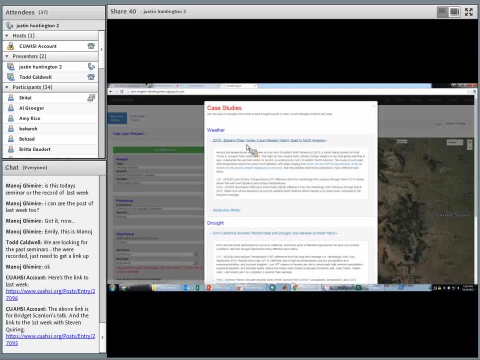 page that you can check out. It hasn't been updated for a little while but related to drought. I'll just show. Oh well, first let's show this: eastern polar vortex 2.. Why 2? Because in 2014 they said the same thing. Let's look at land surface temperature anomaly for this. 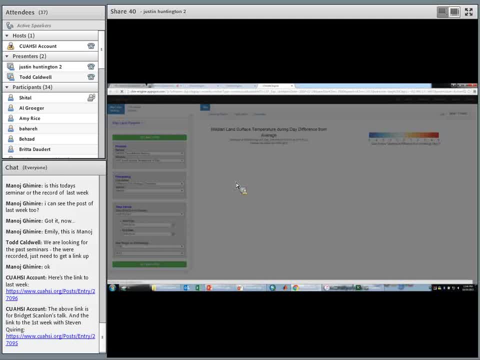 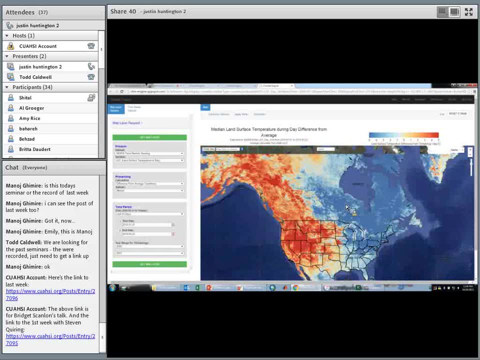 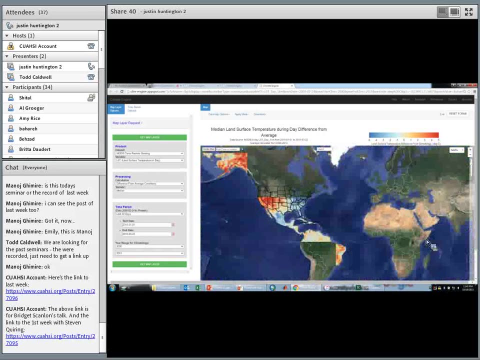 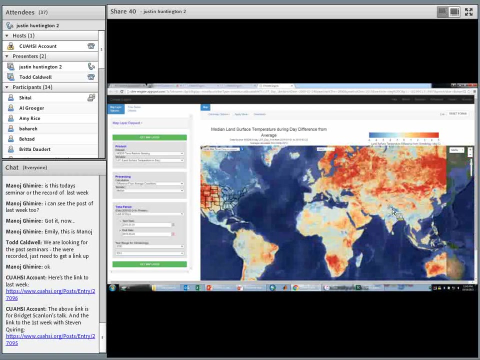 last winter Pretty impressive. It's pretty amazing what we can see here: how warm it was in the west and how just cold it was in the east. And what's beautiful about this is this is a global thing. They have the whole archive. So if you want to start to go global, it's very, very easy to do. 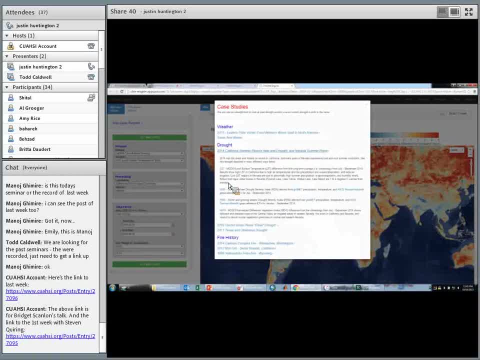 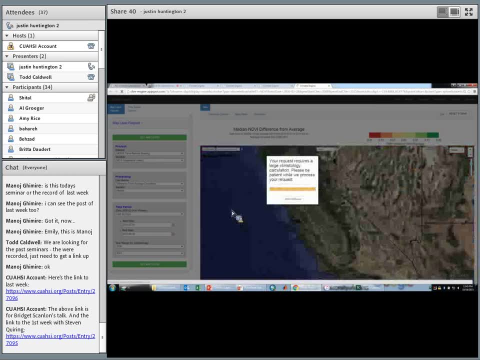 So let's look at some more examples. Let's look at NDVI. Let's take a look at the California drought anomaly. This is focused on the Central Valley. I believe, Yes, Central Valley. So this is last year the NDVI anomaly. So you can see. 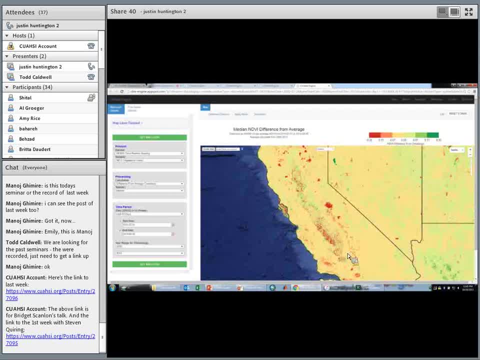 the California drought. No, I didn't pre-run this, So that was not in the cache and that's how this is coming up, using the full archive to calculate the anomaly. Let's do some more examples here. Let's do Texas and Oklahoma. 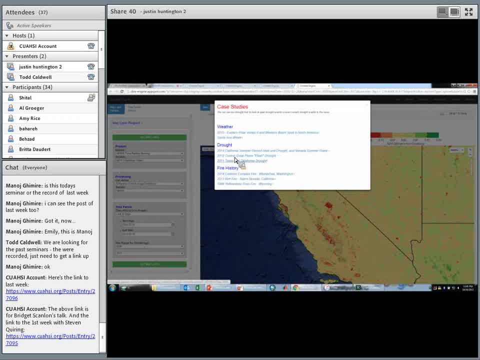 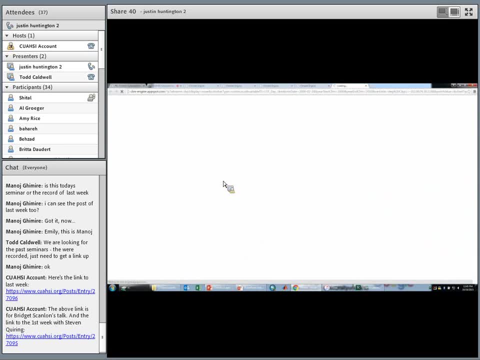 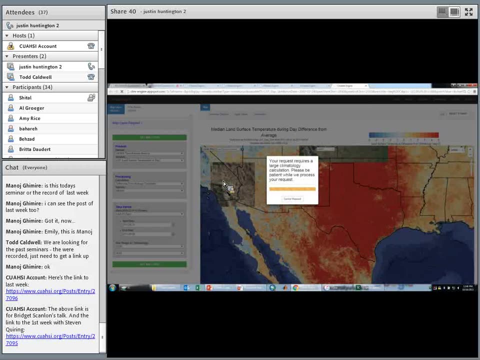 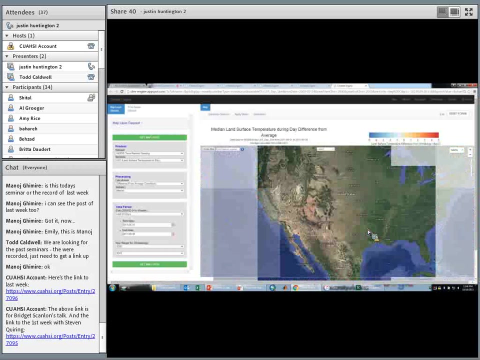 Scot Scot. Scot Scot- Oklahoma Todd since Texas Land surface temperature for 2011,. pretty amazing what we can see here. Of course, this is the big Texas drought in 2011 in Texas and Oklahoma, so pretty neat that that shows up like it does. And then the Central Great Plains flash. 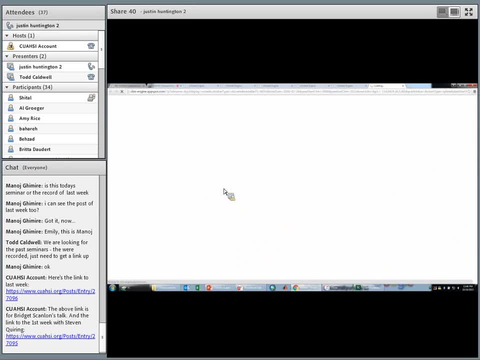 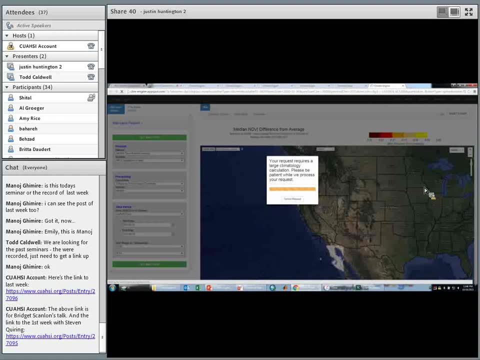 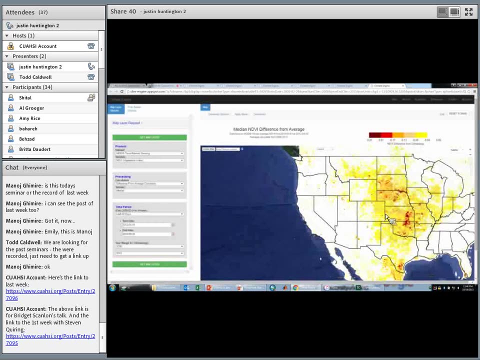 drought. Let's look at NDVI, This difference from long-term average. So yeah, here's that NDVI anomaly for the Central Great Plains: flash drought for the growing season, May through September. Now I'm going to start a new session here. 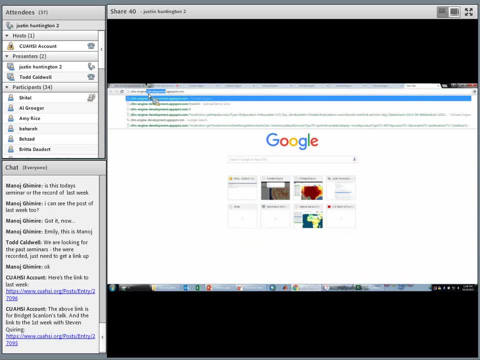 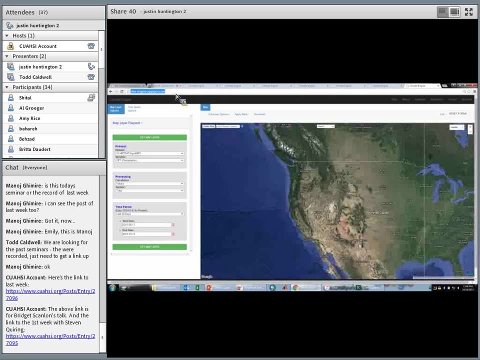 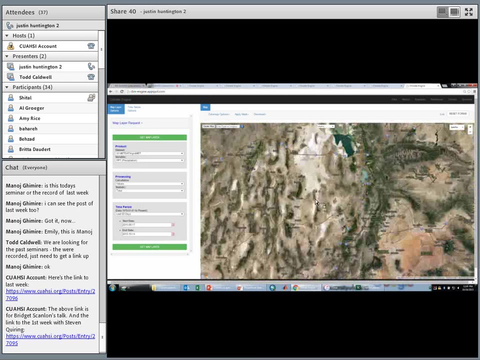 The climateengineorg takes you to our. it forwards you right now to climb-engineappspotcom. AppSpot is the Google front-end web service, But I'm going to zoom in to Needlepoint Spring here, just to show you how you can pull out a time series. Let's see, here I'm a little. 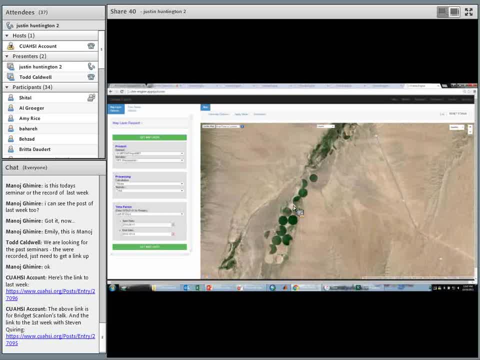 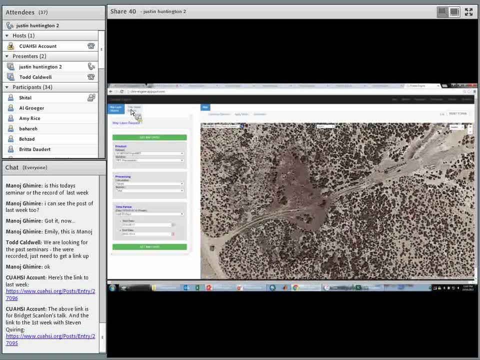 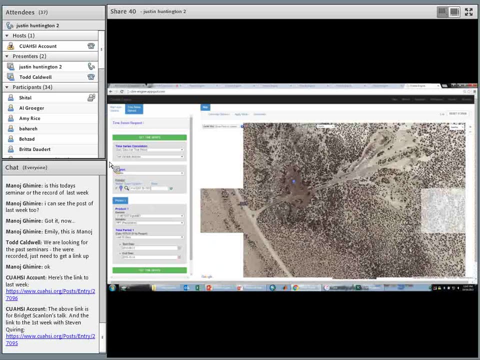 lost. All right, yeah, here we go. So here's this little flip on the map, Needlepoint Spring, and I'm going to click time series and it's going to drop a marker down. I'm going to put my marker right about right there. And daily data, yearly summaries: I'm going to 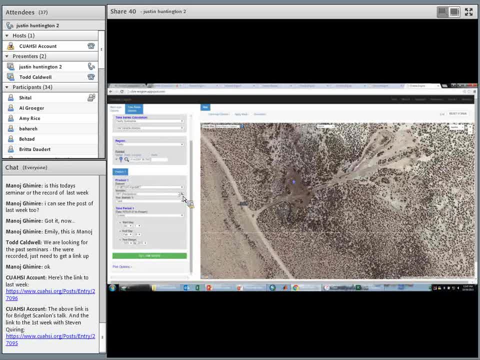 pick yearly summaries and then go to Landsat 5. And I just want to look at the midsummer, August through September. If stuff's still green in August and September, I'm going to do a quick search. You know the roots are getting groundwater So I'm going to set. 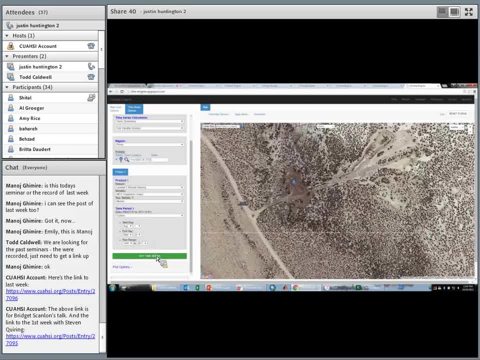 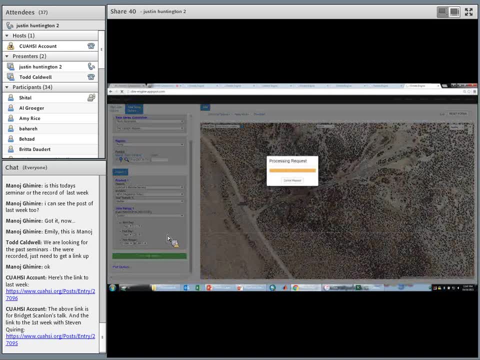 my year range here, Landsat 5, ended in 2012.. So I'm going to say: get time series. We'll cross our fingers if this works. I saw Britta's on the webinar. Britta is the brains behind everything time series on the page, as well as Catherine, But all our plots are developed. 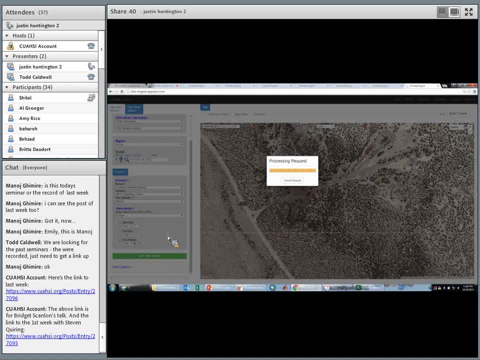 in parts, And so you know I'm just going to put that in there. All right, so I'm going. It's been a bit of a challenge to get everything working well: a lot of JavaScript programming and getting high charts to work. 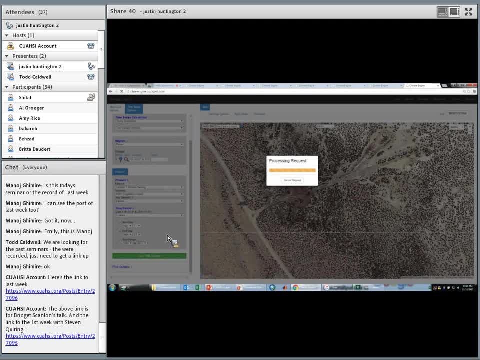 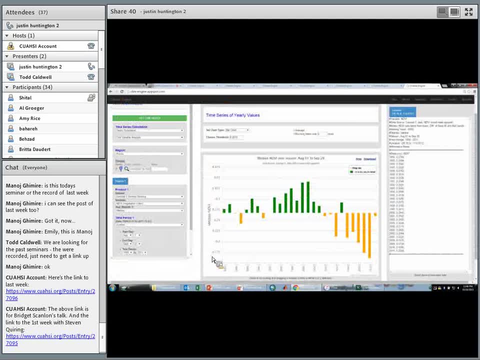 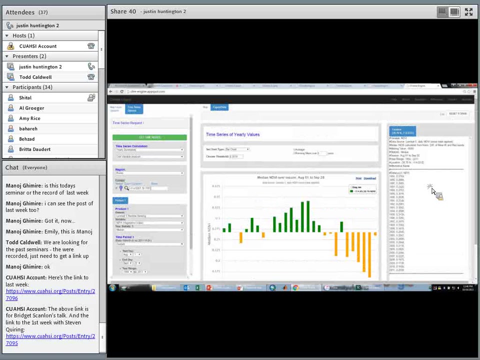 So right now it's computing the median for that date range for every year and you can see that, yep, the spring started to decline vegetation vigor right when the pumping started in 2001.. So, really neat. We print out the time series here that you can grab. 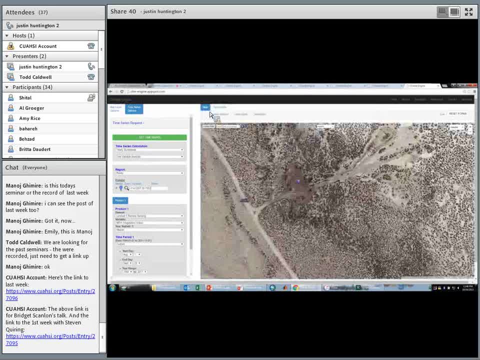 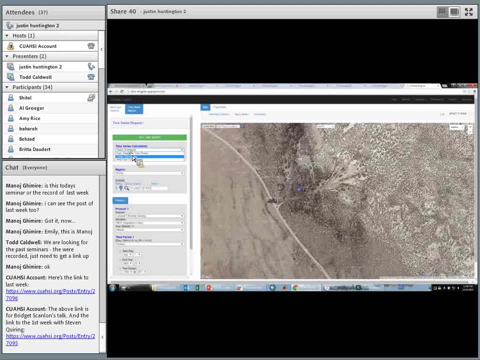 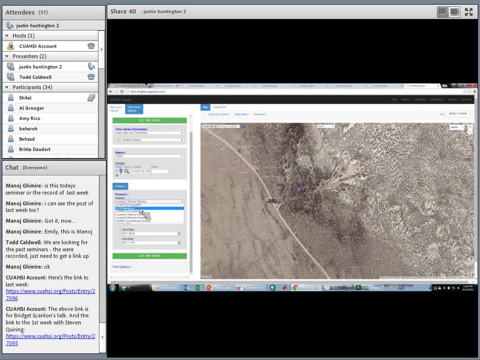 Now, if a lot of people say reference ET for a location, MMO on teeth, reference ET for a particular location. so daily data over time period. I'm going to switch my data set to U of I MET data and then I'm going to pick ASCE reference. 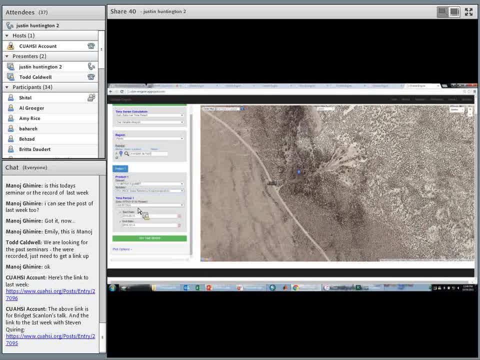 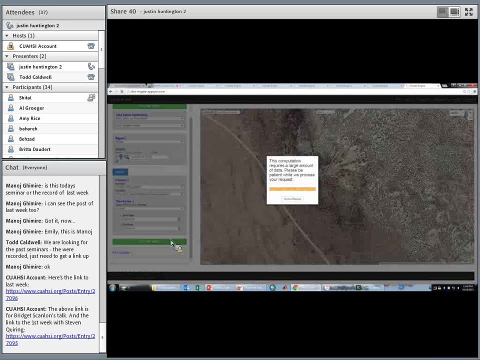 Okay, So I'm going to go to reference ET- grass reference ET- and I want a custom period and say I want like a decade's worth. You can go all the way back to 1979 if you wish- And then it will extract four-kilometer resolution reference ET, Pema Monteith-based reference. 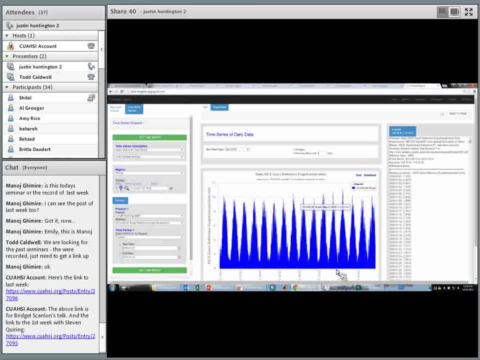 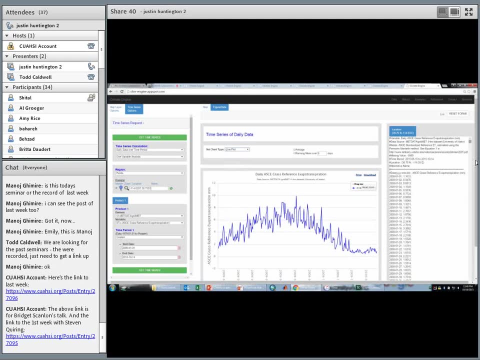 ET and that will be fast. And then you can zoom in and look at particular times, Time series, different types of plotting available, And then, of course, you can get all the data right here to pull into Excel or what have you. You can also share this link with somebody. 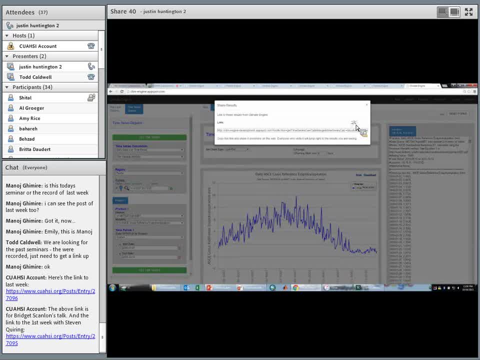 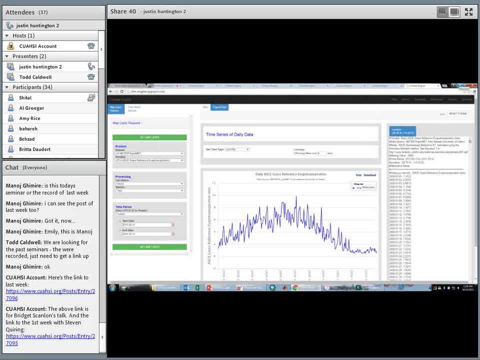 So grab the link and say, hey, check this out, send it to your friend and go from there. So this cloud computing with climate and remote sensing data has just really really changed how we can access data And it's just really really exciting. 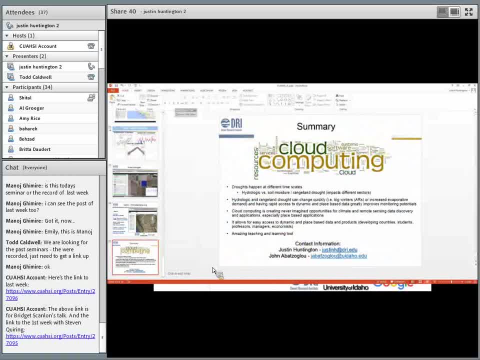 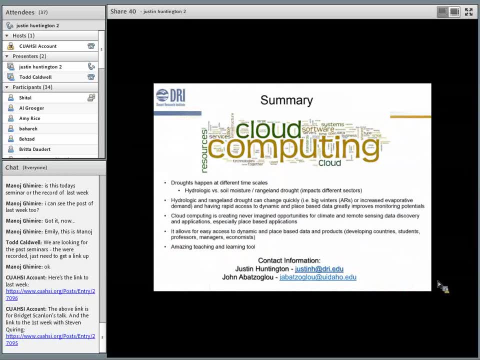 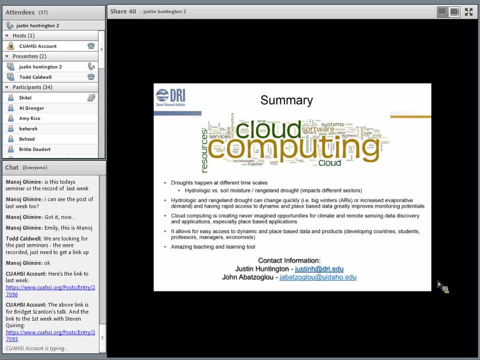 So yeah, with that a little summary here. drought happens at different timescales: Hydrologic versus soil moisture. drought impacts different sectors at a time. So you've got ranchers happy that they found the forage, you've got the irrigators that. 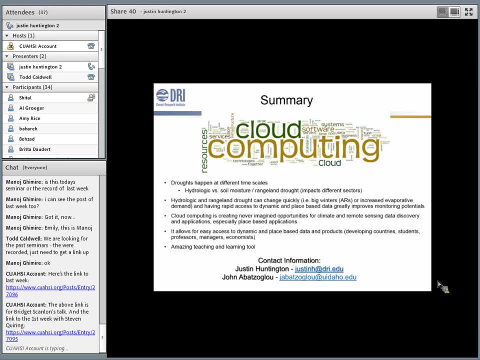 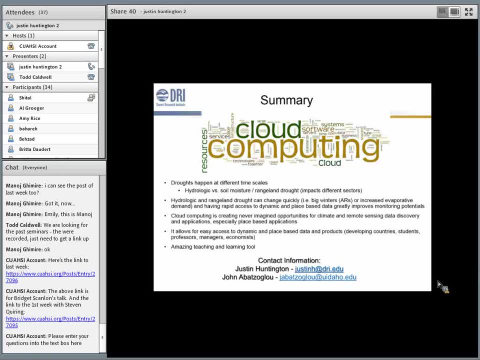 are really sad because there's no water and the BLM that has to kind of manage all this and try to keep everybody happy. So hydrologic and rangeland drought can change quickly. So, for example, if we have a bunch of atmospheric rivers coming in to the Sierra this year, 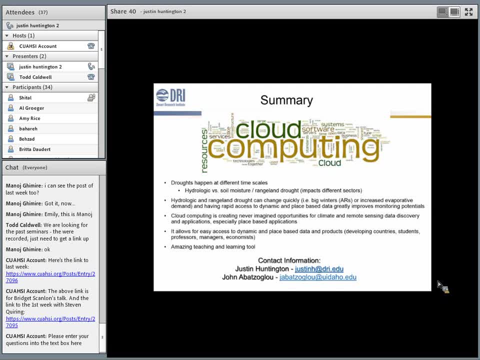 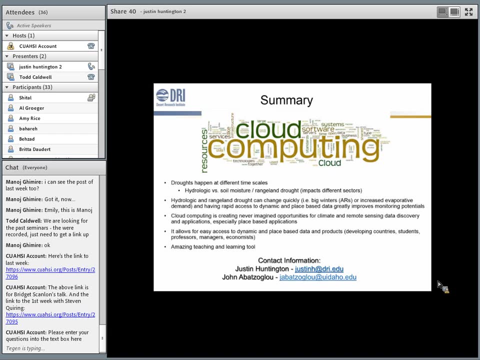 the Tahoe and our Truckee River reservoirs. these smaller reservoirs and systems can fill up fast. On the other hand, we can have really anomalously high evaporative demand and vegetation can dry out really fast, Even though rangeland conditions may be favorable for parts of the year. 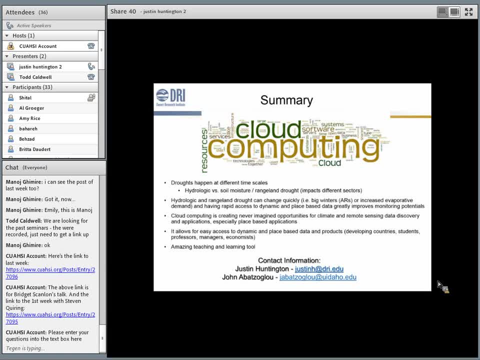 So I'll just note that for bigger reservoir systems, of course, we're going to need many, many wet years in a row, like Lake Mead in the Colorado, to deal with that shortage. But cloud computing is really creating never-imagined opportunities for climate and remote sensing. 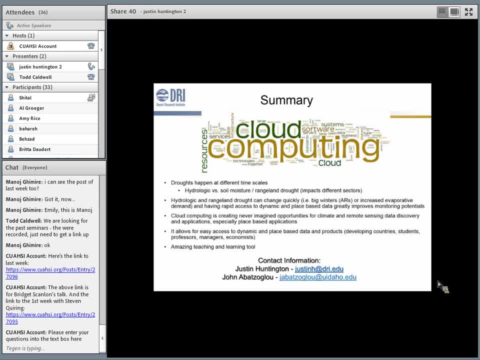 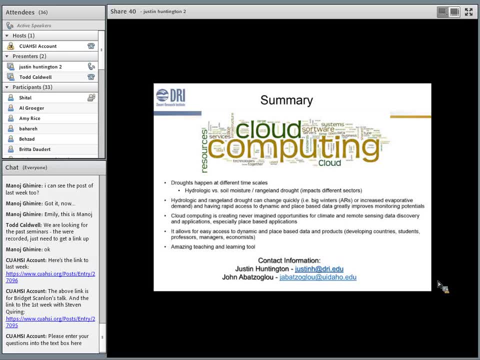 data discovery and applications, and especially place-based applications I mean most. Most maps that use remote sensing right now for drought are very regional in nature. You can't zoom in and look at specific farm districts and pull out times for particular pixels of interest at the 30-meter scale. 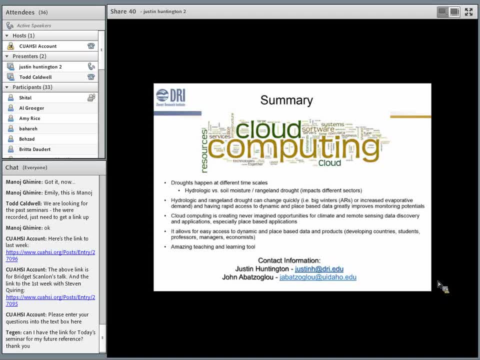 So this is really allowing us tothis new cloud computing and web kind of front end is really allowing us to easily access dynamic and place-based data and products, And this is going to Okay. This is going to be especially useful for developing countries drought monitoring in. 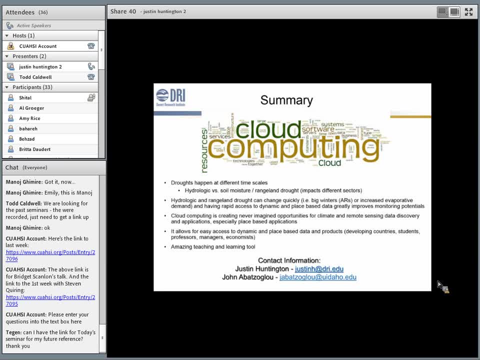 Africa the famine early warning system called FEWS NET group that are now starting to use this technology through our collaboration And it's really helping students, professors and managers and economists and it's really an amazing teaching tool. One thing I forgot to point out that I'll probably get a question about that I need 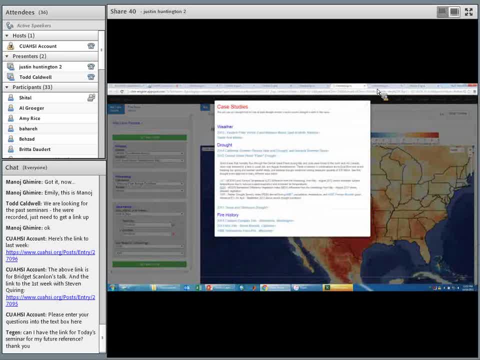 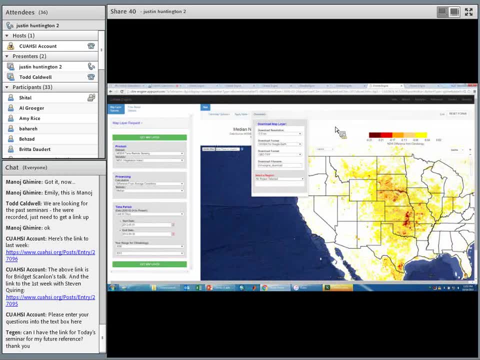 to point out here is that, for example, You can download these results. So that's the thing with this. it's like let's use the cloud computing to generate the results we want and need and then just download the results instead of having to. 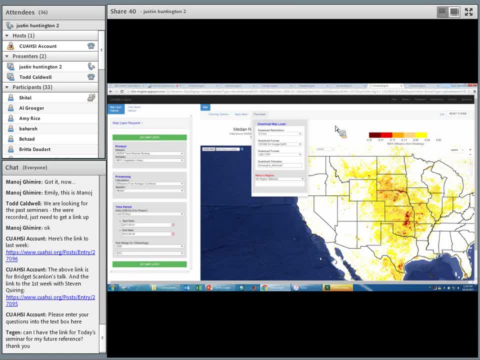 become computer scientists to manage these huge archives. We really, as environmental scientists, just want the dang results, And so you can select download here, Select the resolution you'd like, And then you can just download the results, And then you can use the cloud computing to generate the results. 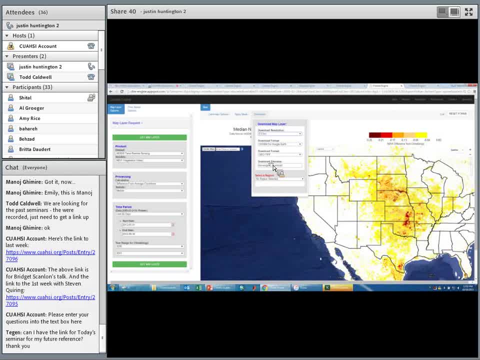 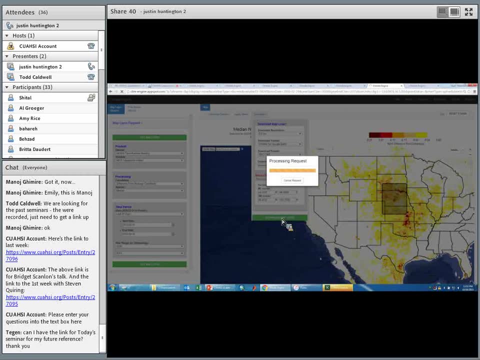 So if I want to do something like GeoTIFF, I'm going to draw a box here, a rectangular region, and so I can go download this NDVI anomaly map. So I'm going to hit download and it's going to clip the result and package it up to GeoTIFF. 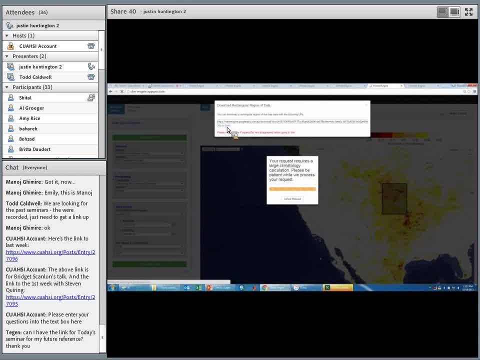 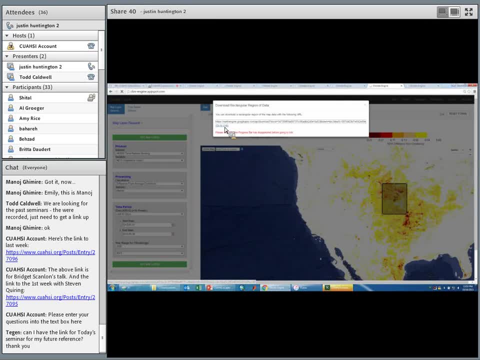 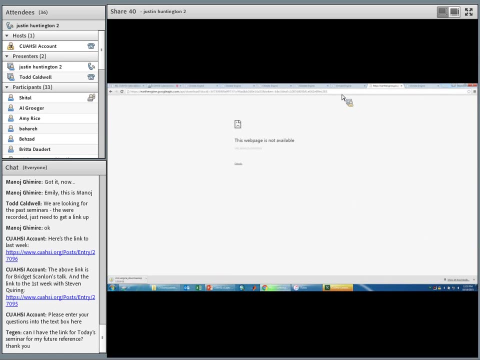 and send me to a link. You got to wait until it's done processing and then go to the link and it'll give me a save as window of the GeoTIFF. Oh, for whatever reason that did not work, But anyways, it typically works. 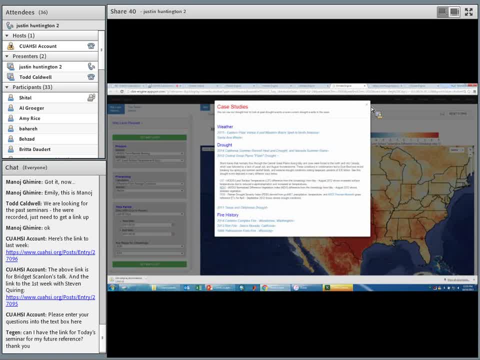 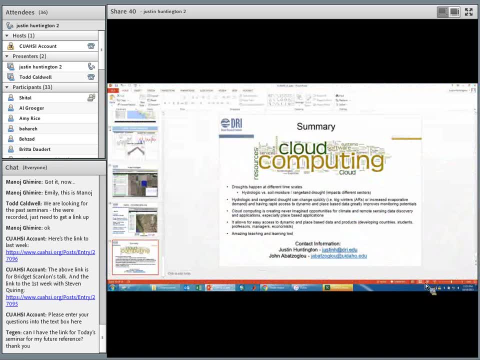 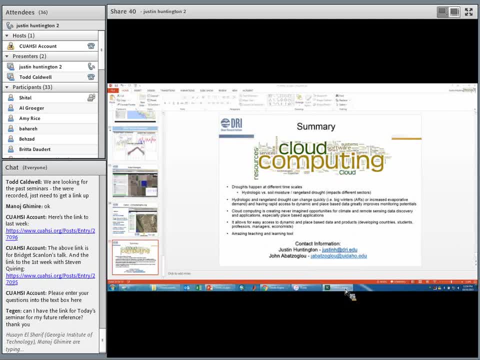 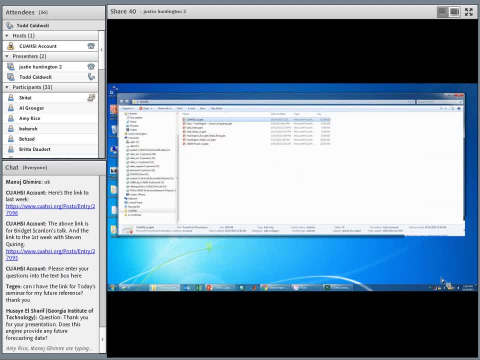 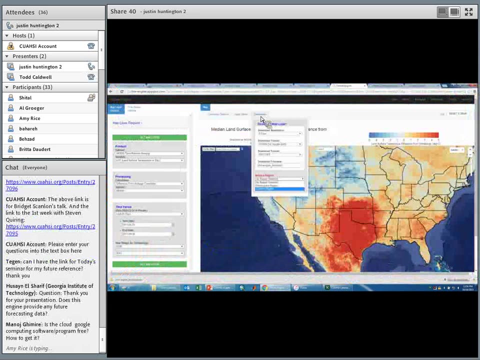 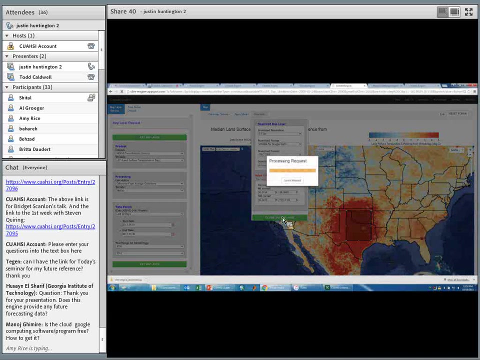 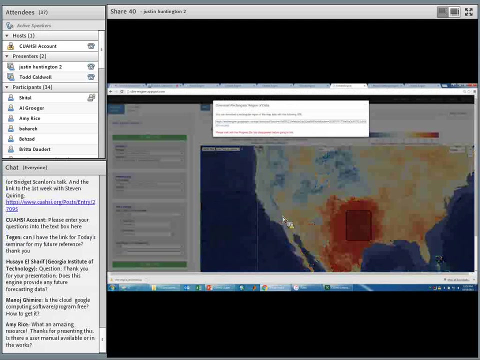 the geotips. what's that? it's always worked. your website has always worked every time. I've gone on there and did you give? okay, I should just add uncommon. yeah, that's inevitable. they would crash during a live webinar. right, let's try to make it happen again. give up yet. yeah, there we go, okay. so here comes some. 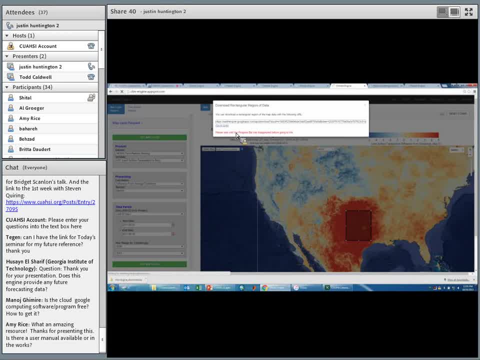 questions: does this engine provide any future forecasting data? that's a great question. we we've worked with Google to put in the maca climate data that it's a downscaled and bias corrected constructed analog type data set. that's that's bias corrected to NLDAS effectively. so it's four. 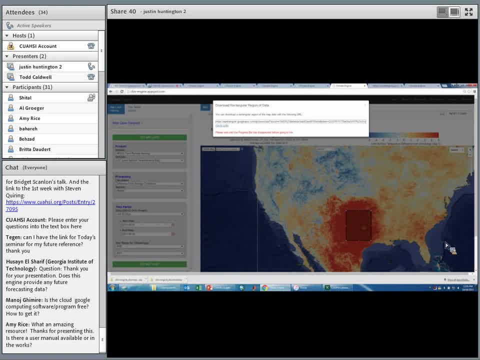 kilometer resolution. it's John Abatzoglou and Katherine's work, and and so that is now in the cloud and we have it ingested into climate engine. it's just that we have those options turned off right now in terms of the data set that we have in the cloud and we have it ingested into climate. 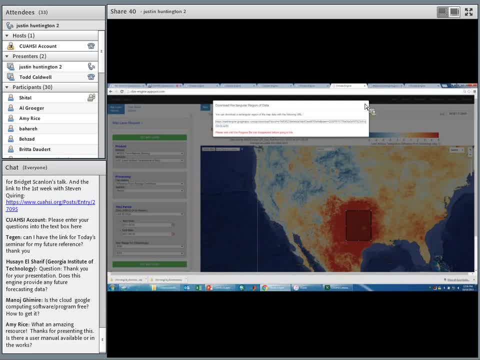 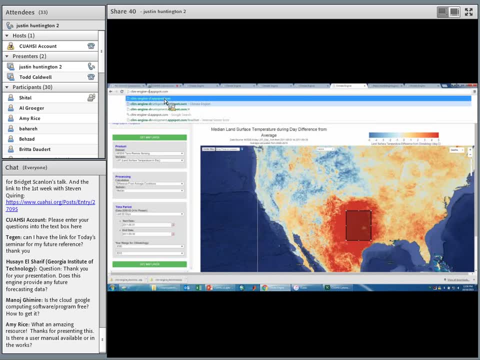 engine. it's just that we have those options turned off right now in terms of the data set that you can select from. so I'm pretty sure we have it off on our development page. if you're ever curious, kind of what we're up to, you can put. 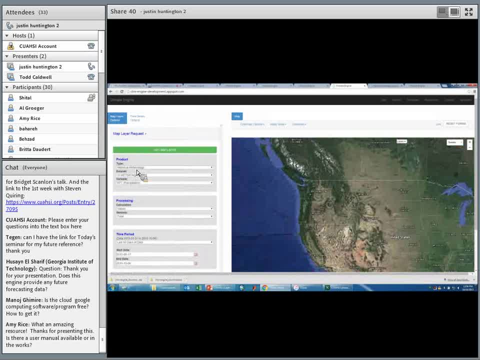 dash development here and go see climate. oh yeah, we do have some future climate. yep, we do have it in there. I thought Katherine had it excluded for a while, but we have the, the, the multi adaptive constructed analog, the UVI data set, and then this NASA next data set, so CMIT five. I've different. 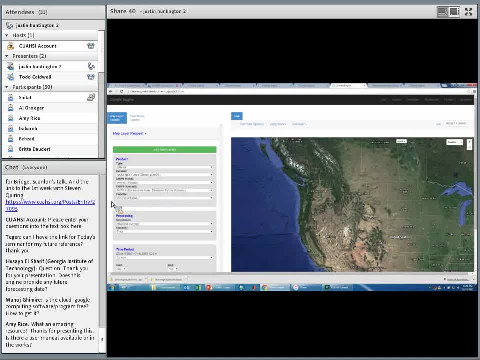 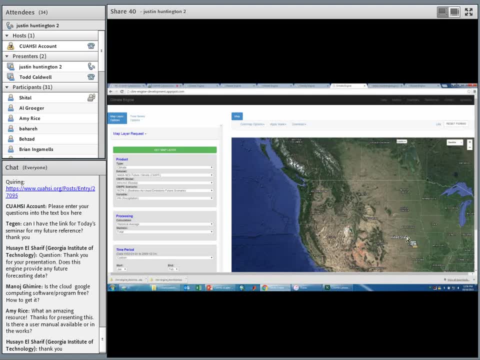 scenarios. that's what going in the future is to be able to: to pull out time-series, maps, our development in terms of testing, like seasonal thing, information and, like in MME type stuff. we're talking about going in, going there, but Google ingested that data set into their cloud. yet is the cloud computing software? 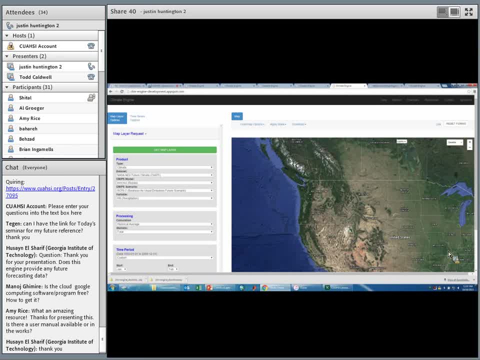 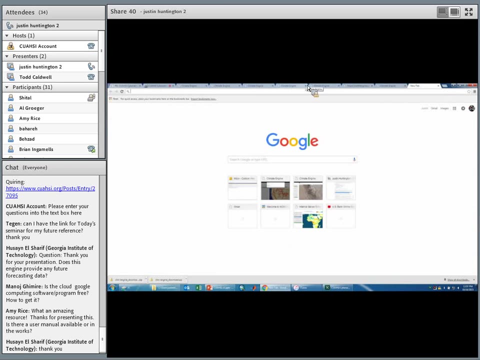 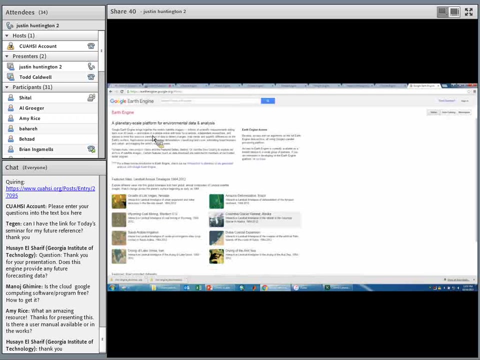 program free. how do I get it? you can sign up for Google Earth Engine. if you just Google Google Earth Engine, you'll go to the page and on the right side, let me just show you how to do it. actually as well, go with Earth Engine. yeah, so if you have seen this page yet, it's, it's fascinating. I just want to. 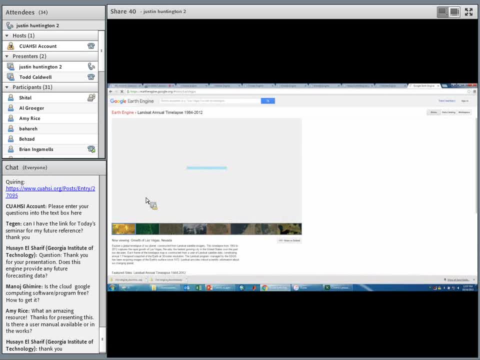 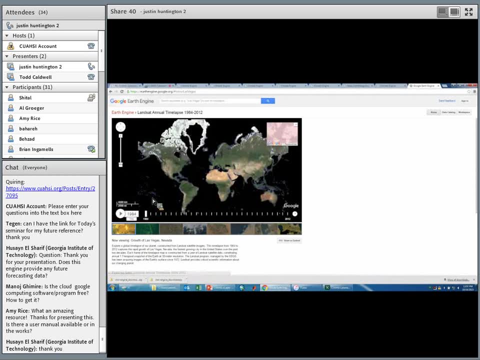 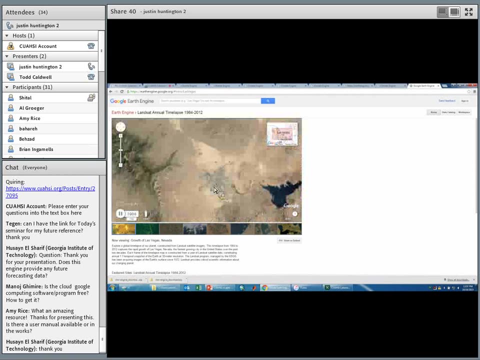 show you this time-lapse. show you where to go, sign up. I know we're getting short on time here, so landsat time-lapse since 1985 anywhere on the planet. so this is Las Vegas growing. but the fascinating thing is is that this is a. 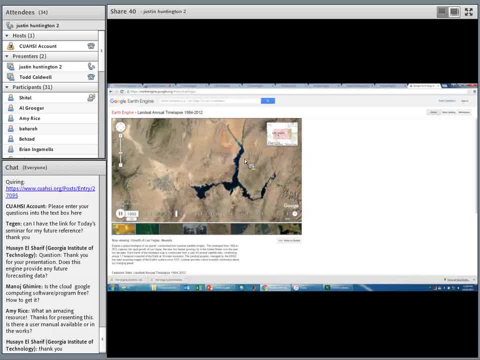 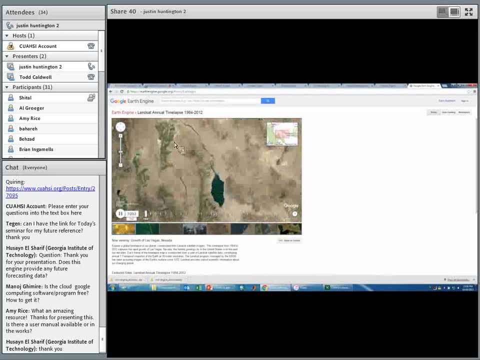 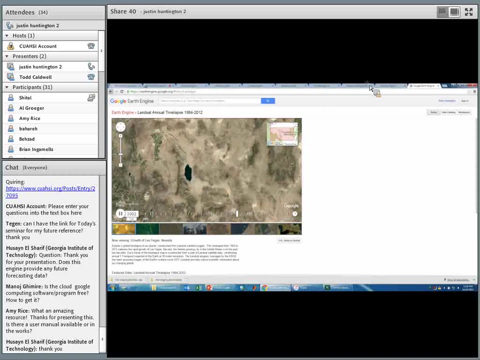 super controlled river and the onlyơi is that's anywhere around the planet. you can see Lake me dropping, you can this Walker Lake here. this is a terminal Lake. all this agriculture in Valley that I highlighted earlier is being diverted and so declining. it's now a dead lake, meaning no fish, because it's salty just. 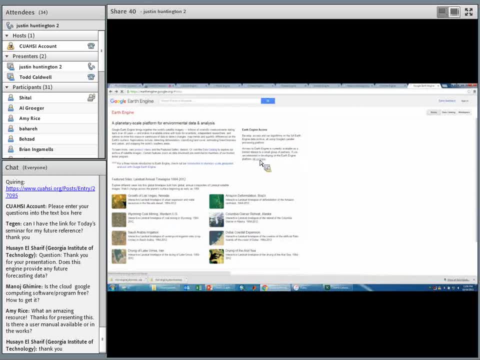 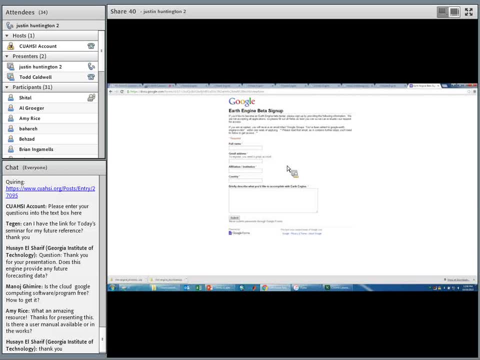 really fascinating. but anyway, let me go back here. so earth engine access. please let us know. if you want to Google Earth Engine engine partner beta sign up. put it here, all your info. they'll give you a link to the playground and then you'll have access to the, to the JavaScript API and 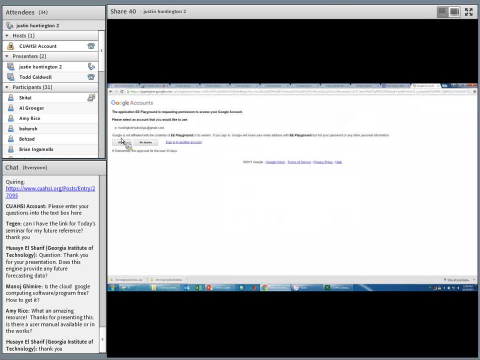 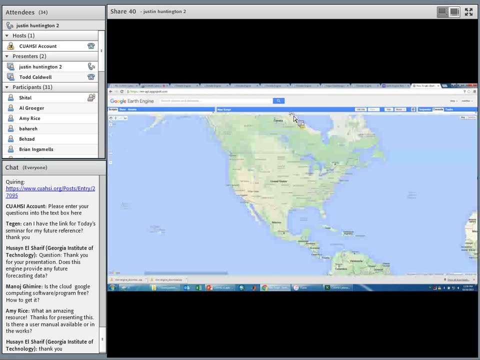 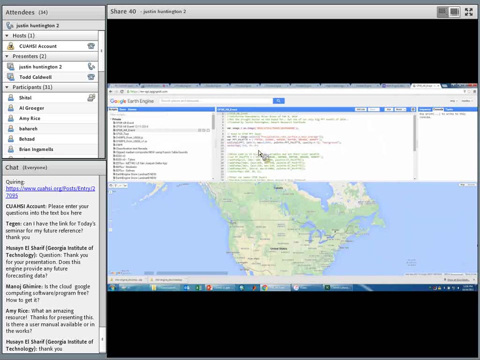 EE app spot: calm and just sign in another account. a lot so the playground where you can code in JavaScript. so this is the CFS our test, where we looked at just testing CFS, our data, making sure it's making sense after they ingested it. so I highlighted a big atmospheric so here 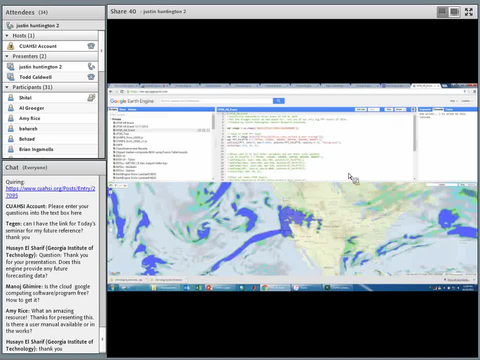 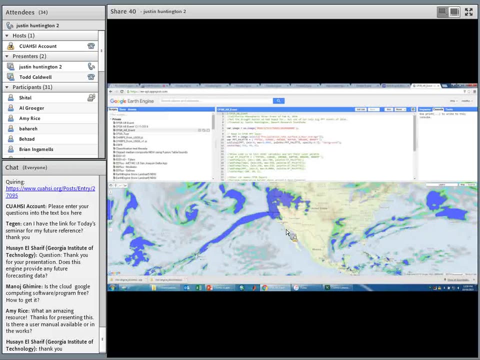 run. it's going to plot precipitation intensity for February 8th of 2014. now this is six hourly data, so this is just as a test. they just ingested CFS, our, So I wanted to see if it made sense, and so I focused in on what I knew was a big AR. 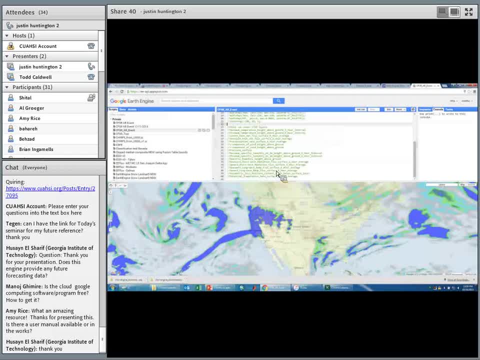 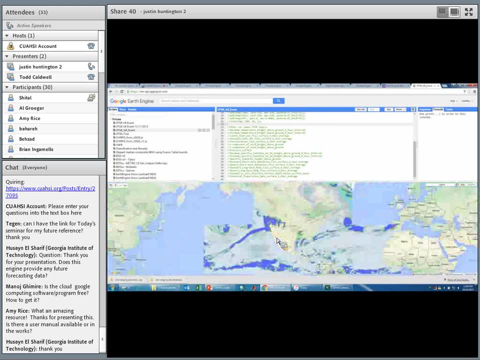 So that's pretty neat, But it's all JavaScript. Within CFSR, you know, we have all these different variables: latent heat flux, sensible heat flux, It's global, It's, you know, over the oceans, which is really neat. 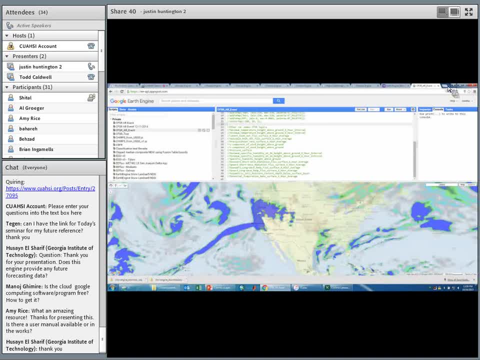 So once you get access to Earth Engine, this is what you get access to. basically, is this Python or JavaScript API called the Playground- Let's see question- an amazing resource. thanks for presenting. Thank you, Amy, And more thanks. 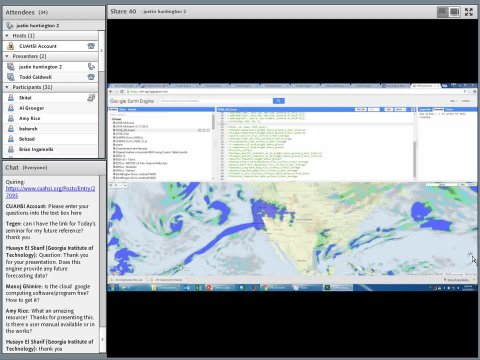 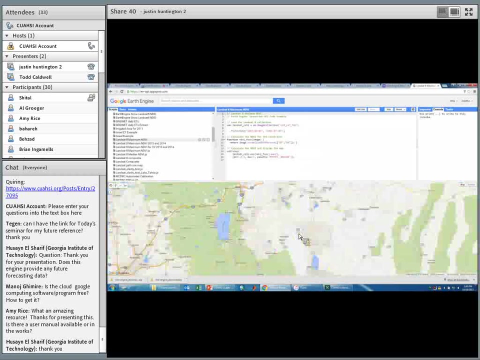 So I think that is all I see for questions, and it's exactly 1 o'clock, so perfect. Any questions from anybody else? or you, Todd, or Emily? No, thank you. Thank you for the presentation, very interesting and slightly concerning. you know the trends. 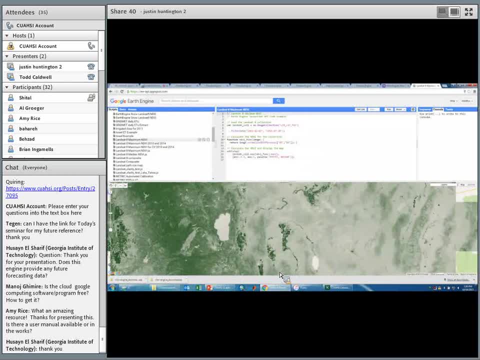 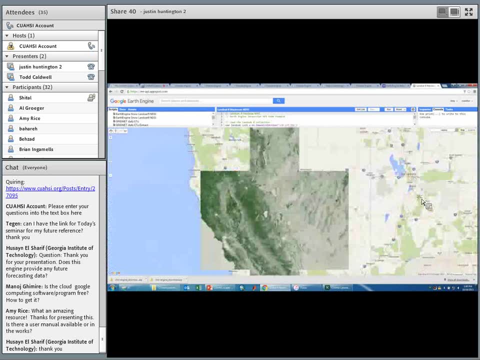 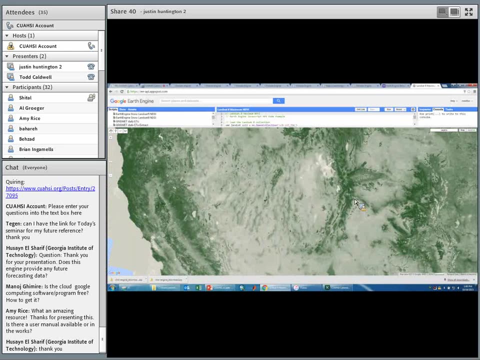 that are going on. I do want to remind all the participants that we have another speaker next Friday at 3 pm and that will be Brian Fuchs, from the Drought Mitigation Laboratory at the US Department of State at University of Nebraska. 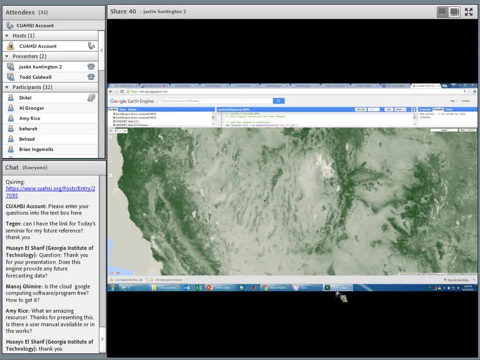 But that's it. I just wanted to remind everyone of next week's talk, and we'll be staying on the theme of drought. Yeah, thanks, Justin, and thanks Emily for all your help. Oh, yeah, Yeah, and thanks everybody for your interest in the topic and I hope to see you next week. 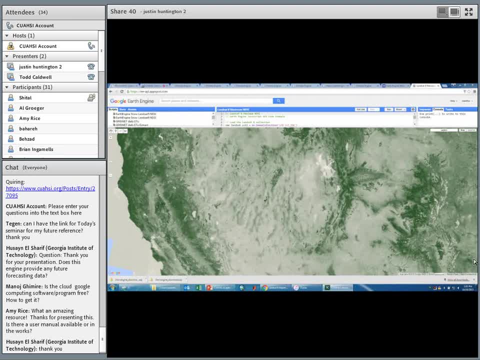 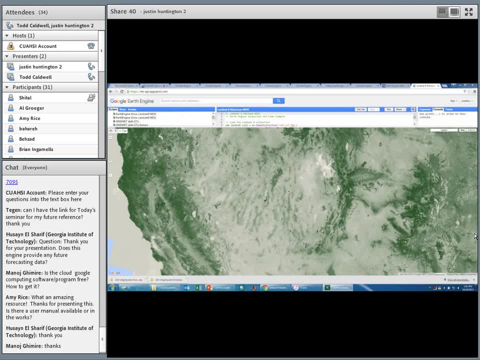 Thank you. Thank you, Thanks, Justin, and if you have any questions or want to know more about this stuff, feel free to email us. Thanks again, All right, Thanks Justin, Thanks everybody.